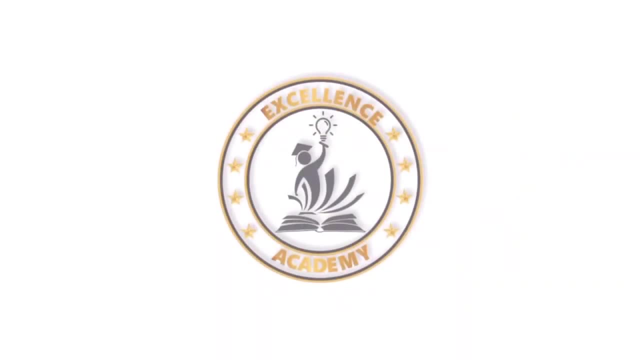 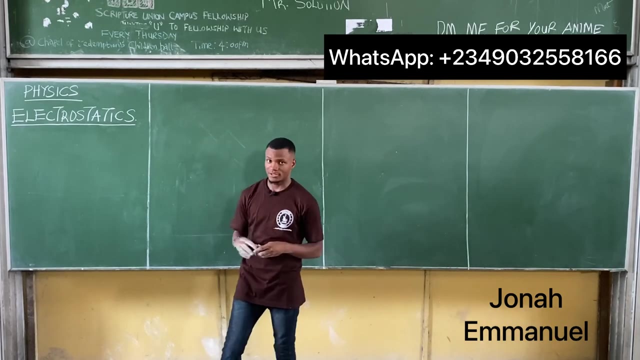 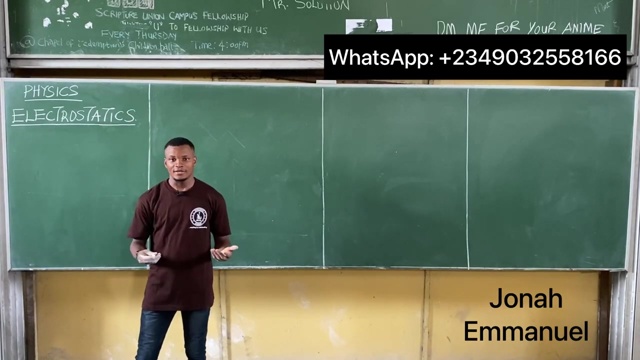 Hello and welcome to today's class, For today we will be looking at electrostatics. Now let's start with the main definition. By definition, the term there is electrostatics, right. Electrostatics is actually a compound term that consists of two words: electro and statics. Electro talks about electrons, or perhaps charges, while statics talks about something not moving. alright, That's really just a particular position. 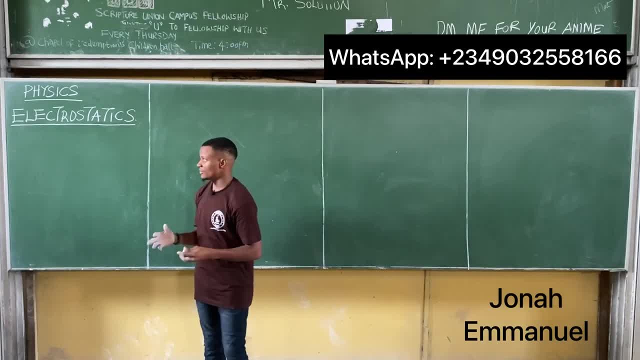 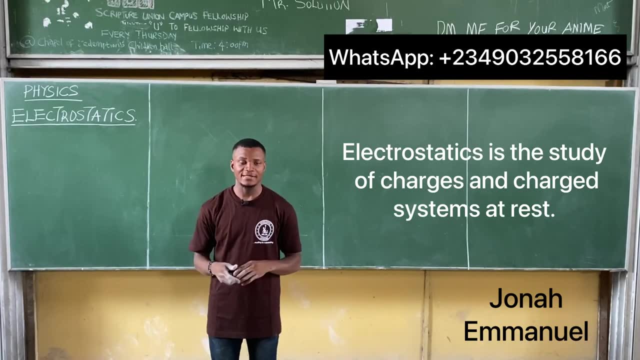 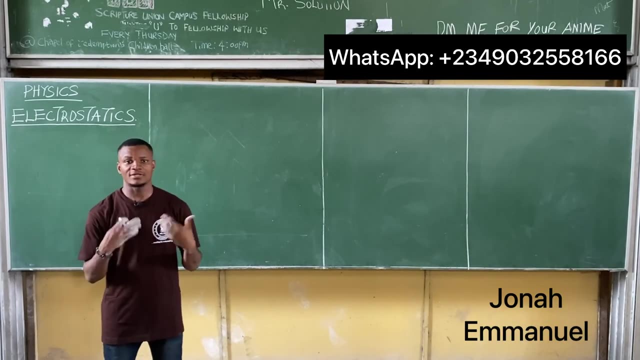 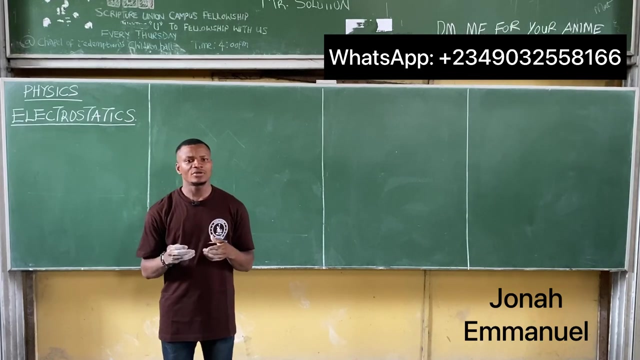 If I combine these two definitions, we can define electrostatics as the study of charges and charge system at rest. That's the basic definition for electrostatics. Now, aside that, there's a broader view of electrostatics, And in this broader view we can consider electrostatics as considering charges that are not just at rest but also moving with a small velocity, or perhaps moving slowly. 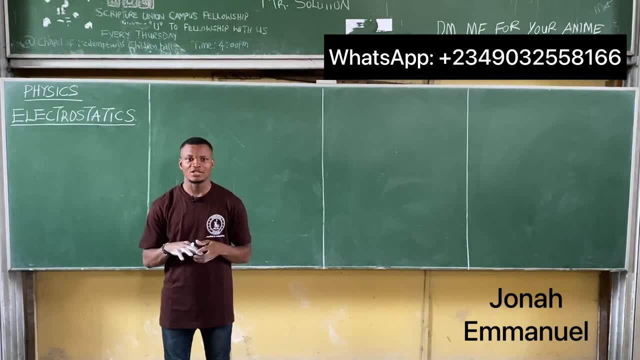 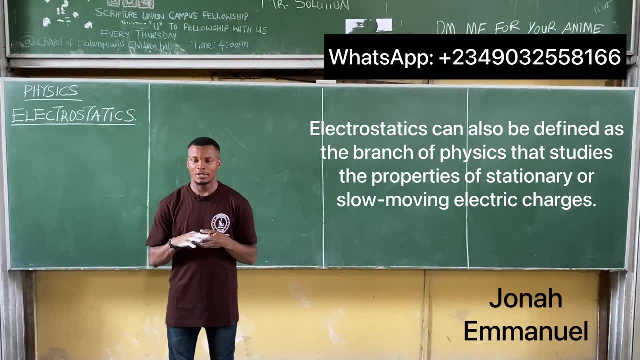 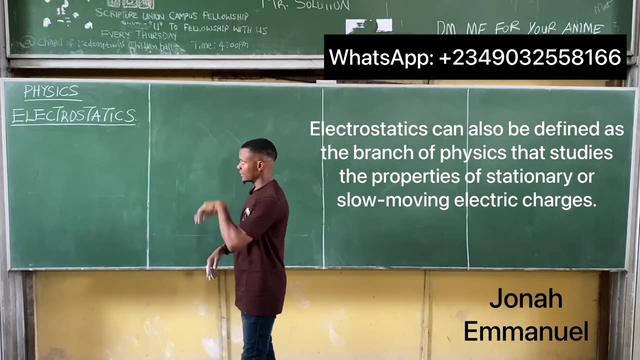 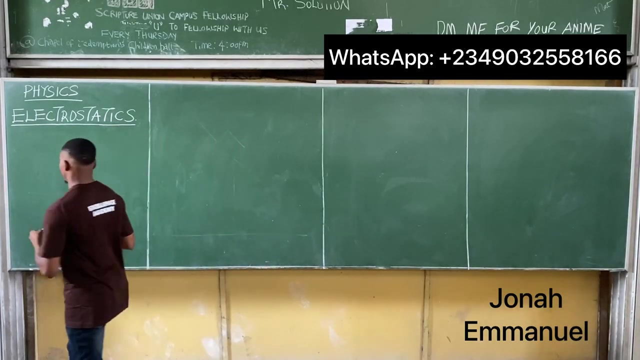 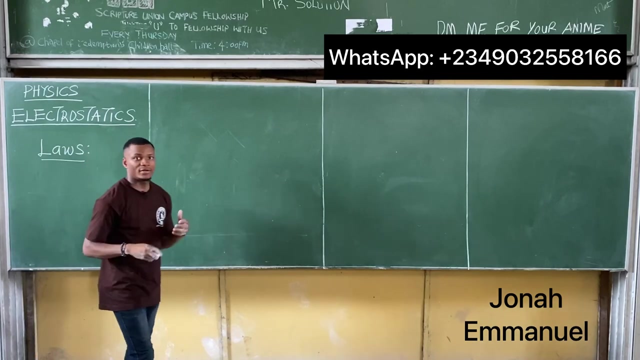 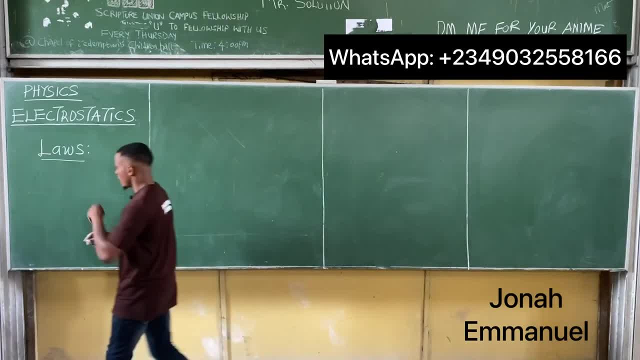 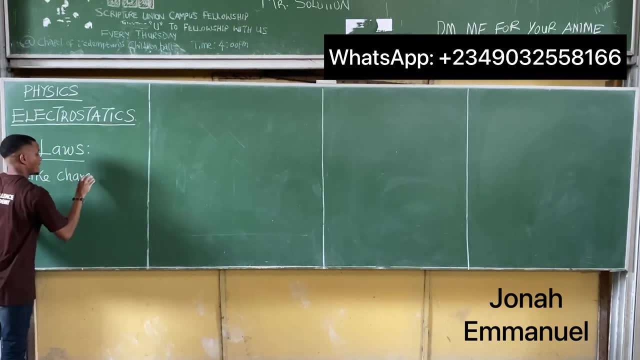 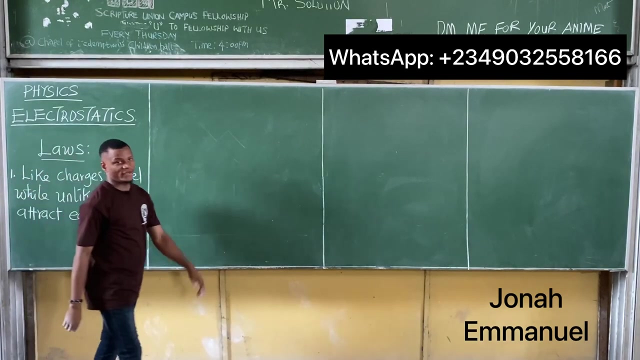 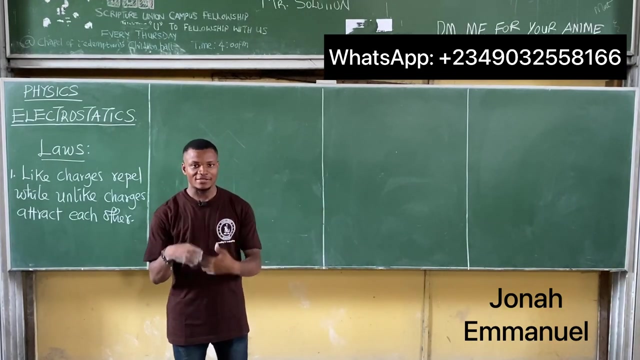 The first law states that light charges- light charges repair, while on light charges attract. Alright. this becomes the first law of electrostatics: Light charges repair, while on light charges attract. So if I have a positive and a positive charge being brought to each other, they will repair, alright. 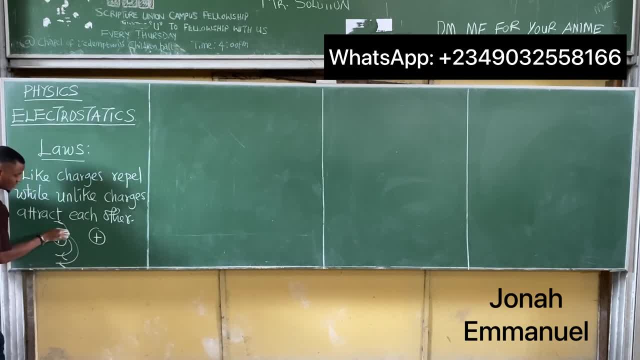 This is how we show repulsion. alright, They will repair. This is showing repulsion. So, as you can see, here there are the same charges, so they will repair Similarly to negative charges. if I bring two negative charges, they will repair as shown like this: 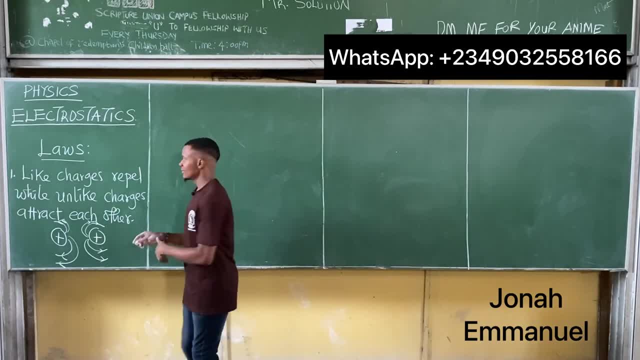 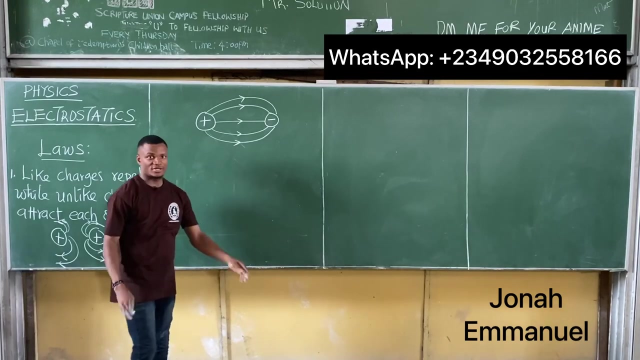 But if I bring a light and an on light charge- let's say a positive charge, on course, and a negative charge- an attraction will take place. You have this, They will connect like this. So you have an attraction. There is usually an attraction between all light charges: positive, negative. 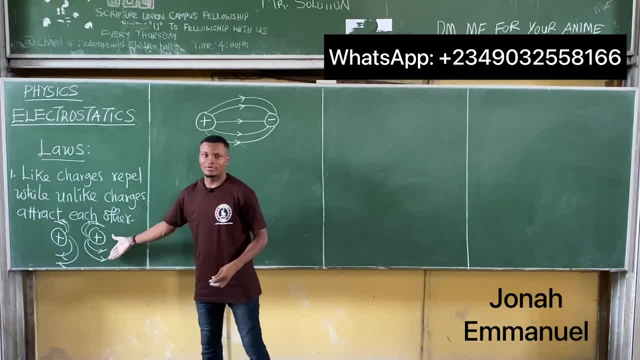 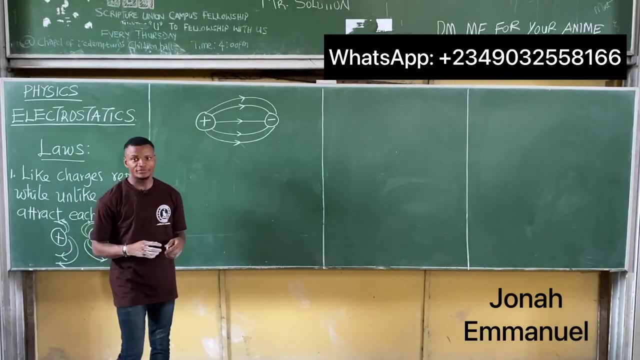 And, of course, a repulsion between light charges, either positive, positive or negative, negative, Alright, so this is the first law of electrostatics, Alright. important to note is the fact that, when it comes to what I do is, 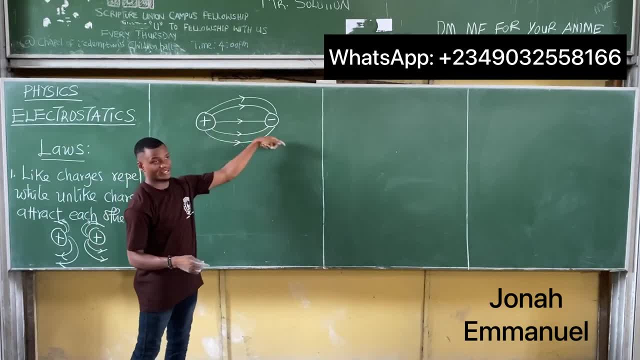 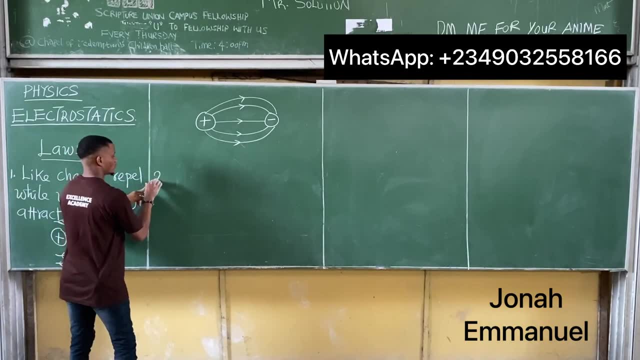 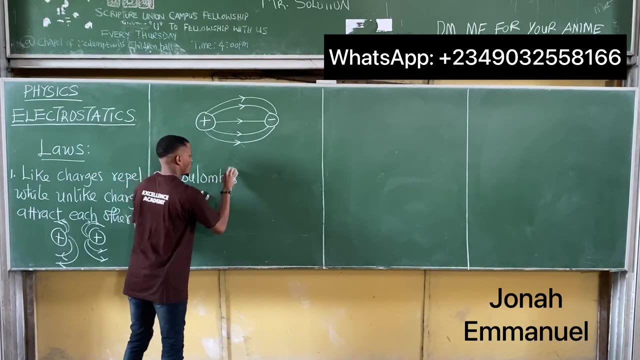 that my direction is from positive to negative, Very important to note. So that's the first law of electrostatics. The second law of electrostatics is also called Coulomb's law. The second law of electrostatics is also known as Coulomb's law. 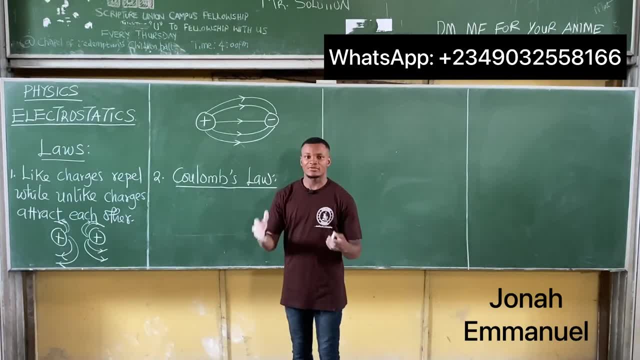 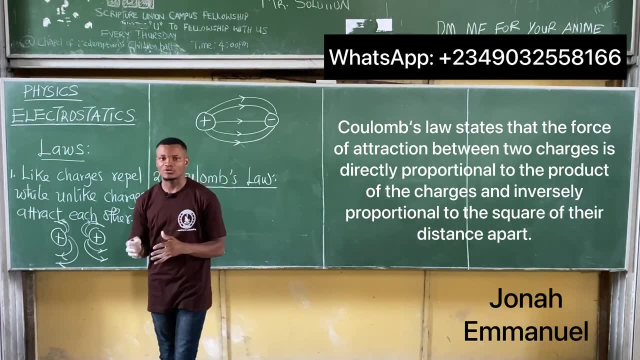 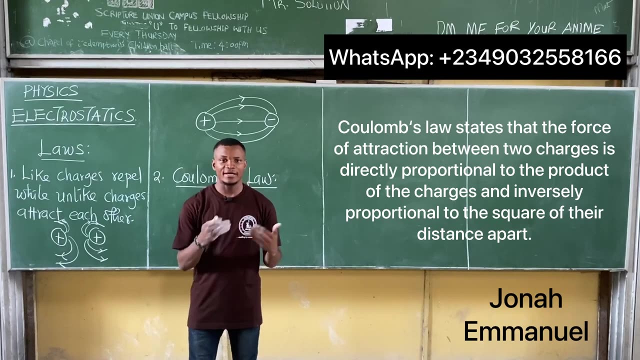 Coulomb's law states that the force of attraction between two charges- let's say Q1 and Q2, is directly proportional to the product of the charges and inversely proportional to the square of their distance apart. Alright, In mathematical terms, let's say: I have two charges. 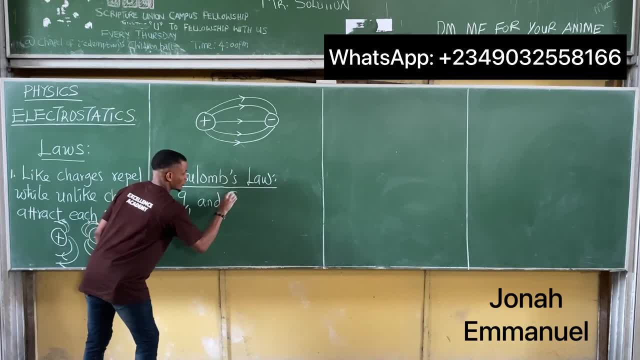 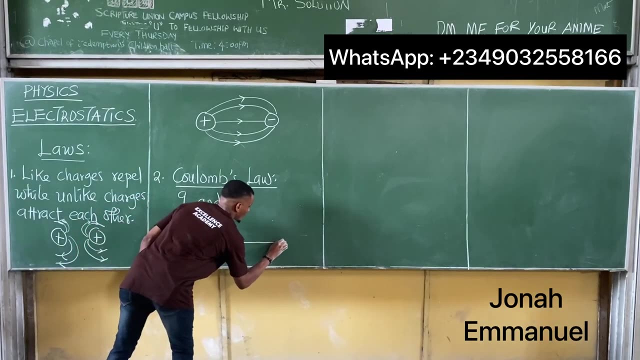 Let's say Q1 and Q2.. And let's say these two charges are separated by a distance- I don't need a diagram to demonstrate this. So I have charge 1.. So I have charge Q1 and charge Q2.. 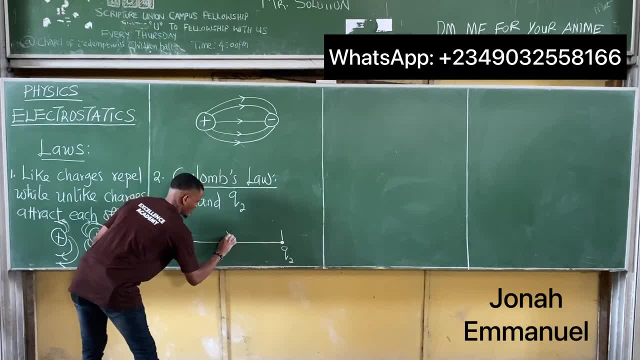 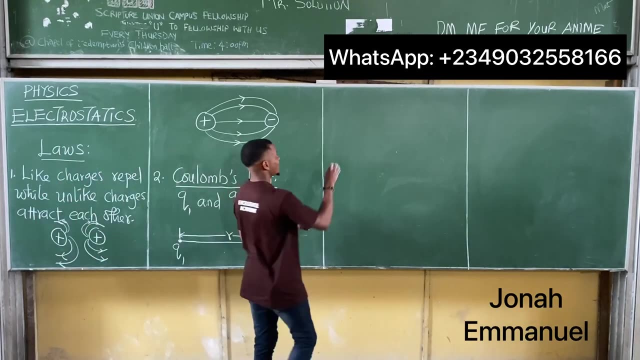 Here and here This becomes I. Alright, So let's say we have two charges, Q1 and Q2, separated by a distance, I. We said from Coulomb's law that the force of attraction between the two charges, the algebraic terms. 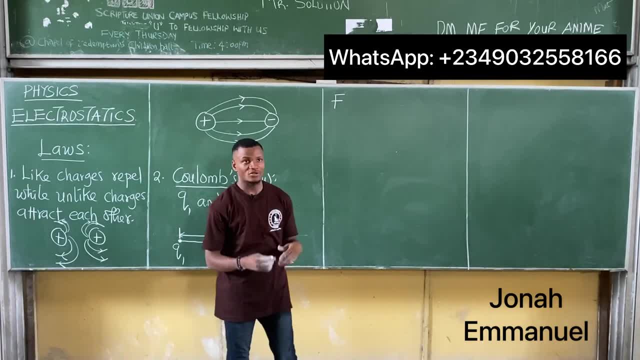 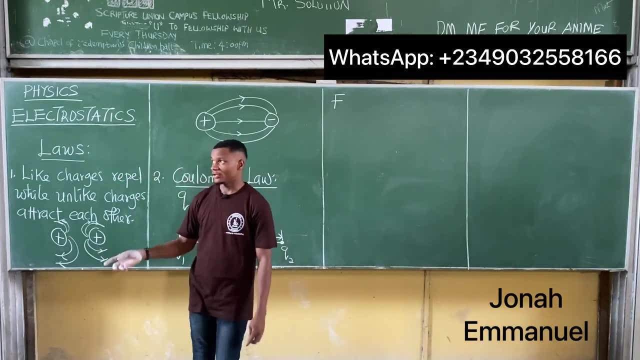 So we are saying that the force of attraction. of course we can also say all repulsion, because if the charges are the same, they will repel, If they are opposite, they will attract. So we said the force of attraction, all repulsion, all repulsion. 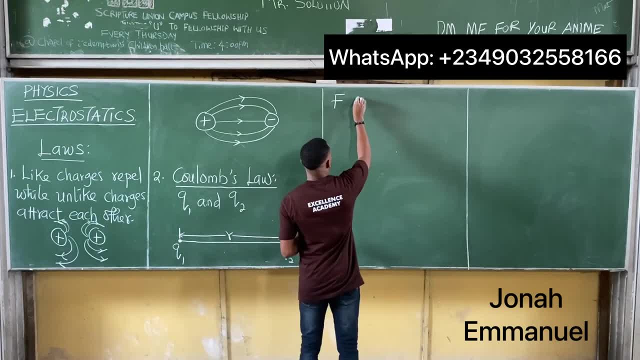 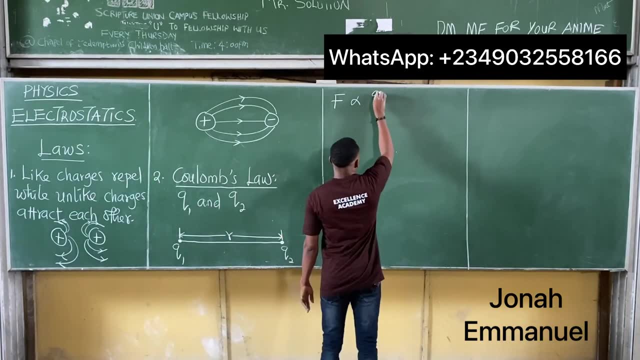 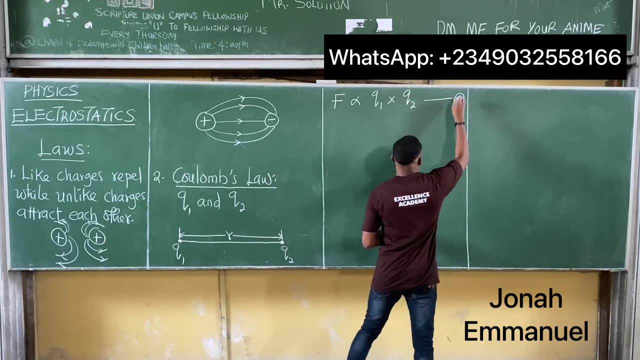 between two charges is directly proportional to the product of the charge. Here I have Q1 and Q2 to become. Product means multiplication. It becomes Q1 times Q2.. That's the first equation I will say. and it's also inversely proportional. 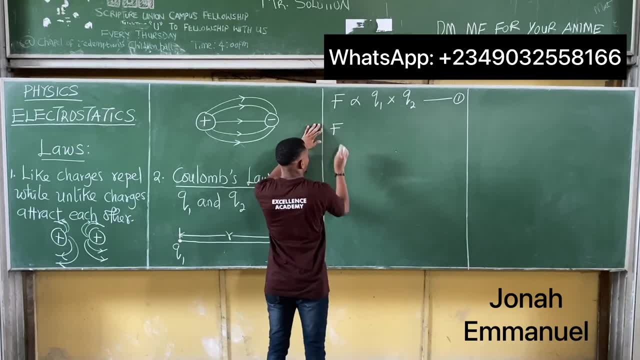 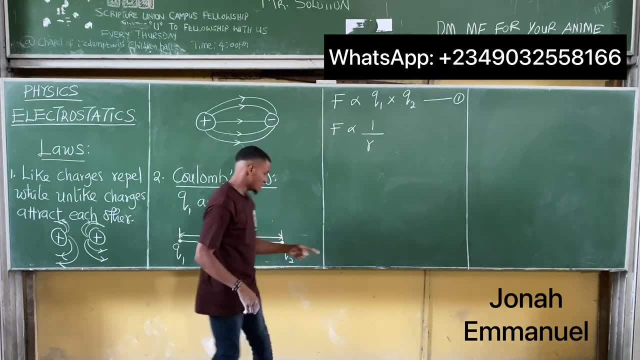 To show inversely proportionality, inverse proportionality. we'll take this as 1 over R, Now it's inversely proportional. It's inversely proportional to not just the distance apart but the square of the distance apart. So very important. 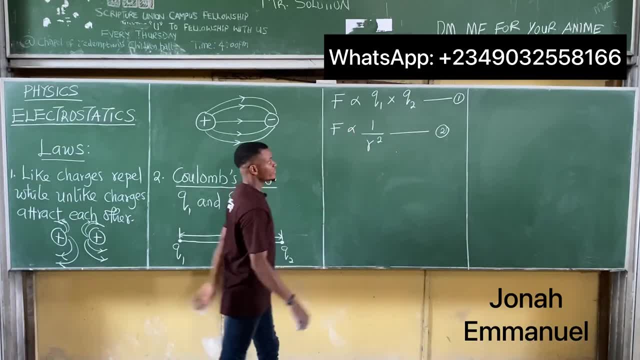 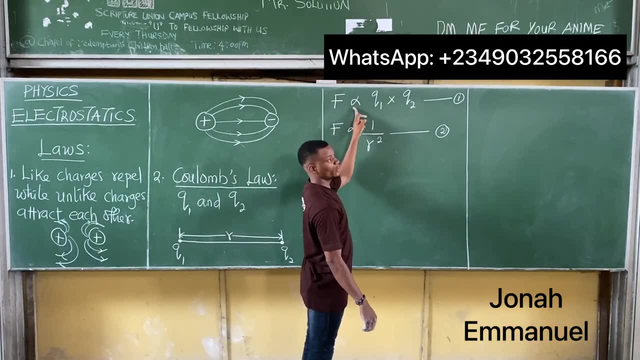 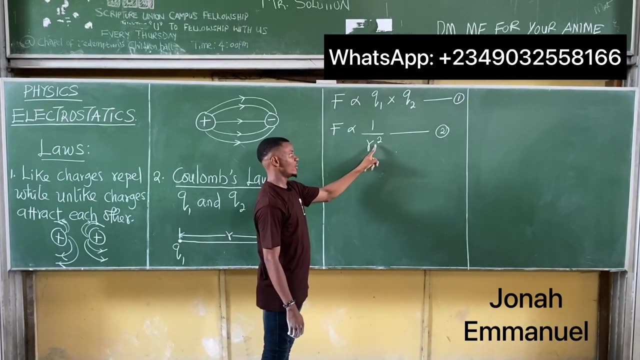 This becomes square. So this is Coulomb's law. in mathematical expression, The force of attraction between two charges is directly proportional to the product of the charges and inversely proportional to the square of the distance apart. Combining 1 and 2,. 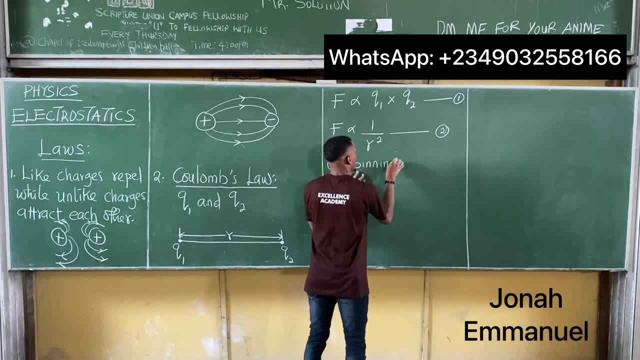 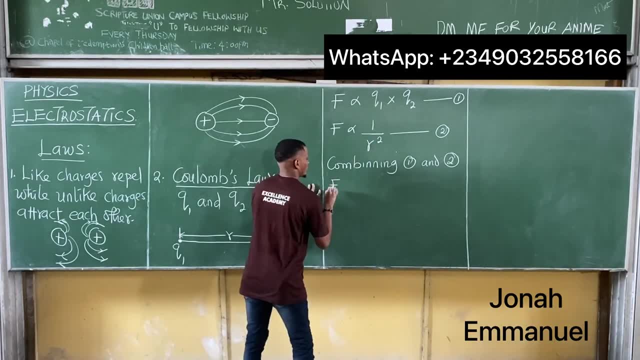 combining 1 and 2,. if I combine 1 and 2, I have that F is directly proportional to Q1- Q2.. Q1- Q2 means Q1 times Q2.. And inverse, proportional to R squared. So I have this: 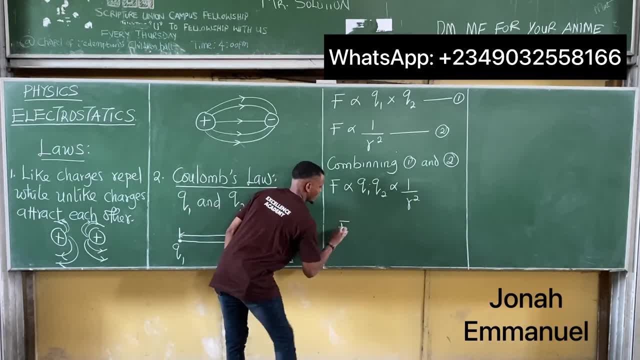 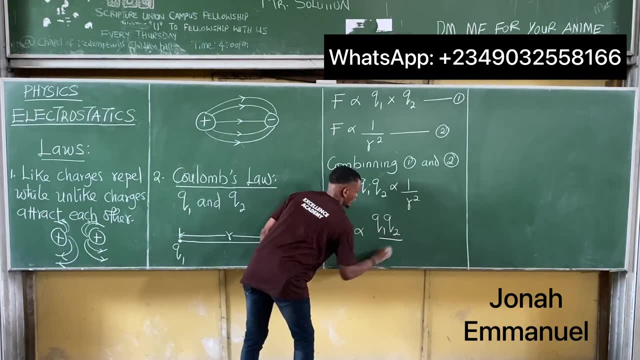 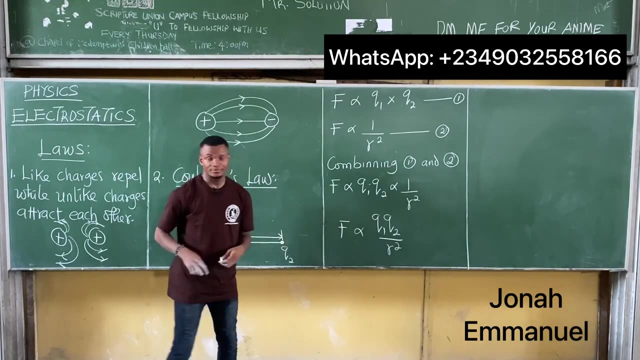 Alright, Combine all of this. It means that F is directly proportional to this 2. It goes to the numerator That gives you Q1, Q2, all over. This one here gives you R squared. So I have this, And of course, again. 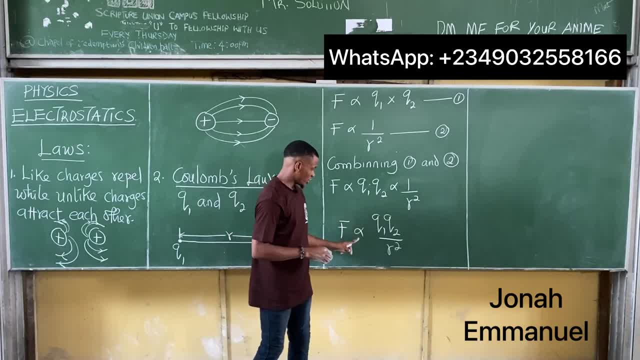 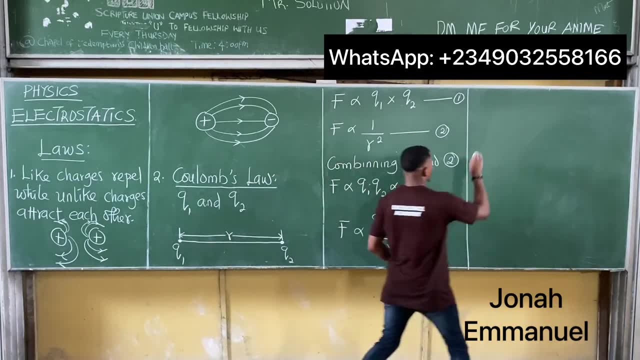 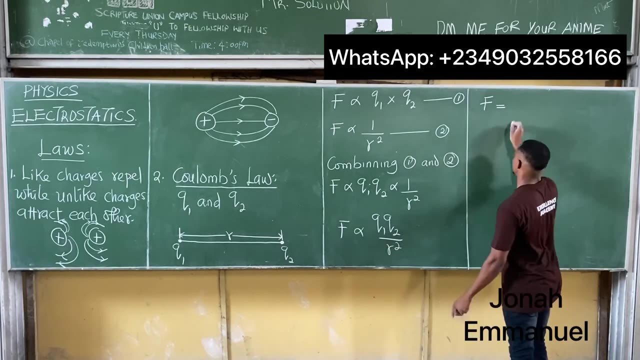 from mathematical approach, we know that to tick off my proportionality sign, I'll introduce an equal to and a constant. So in this case, F, this will now be replaced by an equal to and a constant. The constant in this case is K. 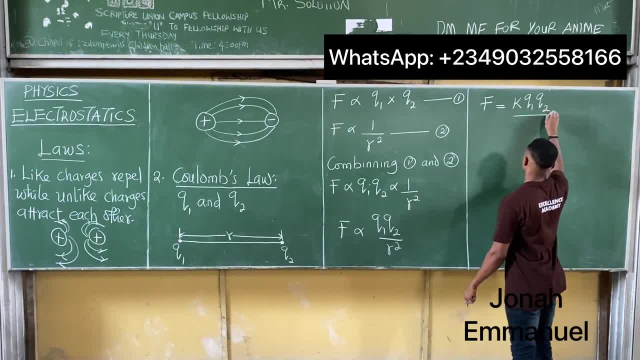 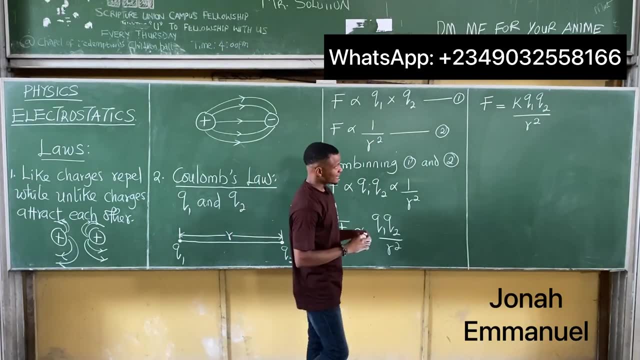 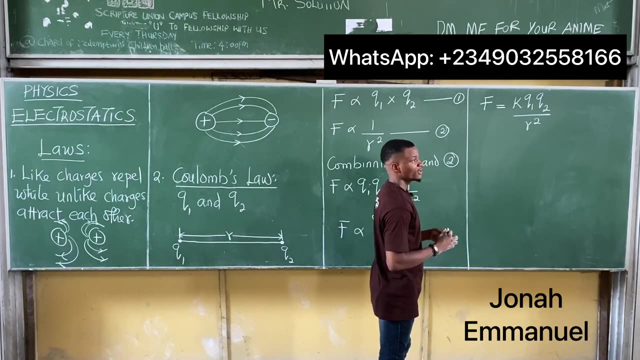 So K, Q1, Q2, all over R squared. So I have this expression Alright. So what next? Let's get the end sign of K. Let's make K the subject of the formula. This becomes all over 1.. 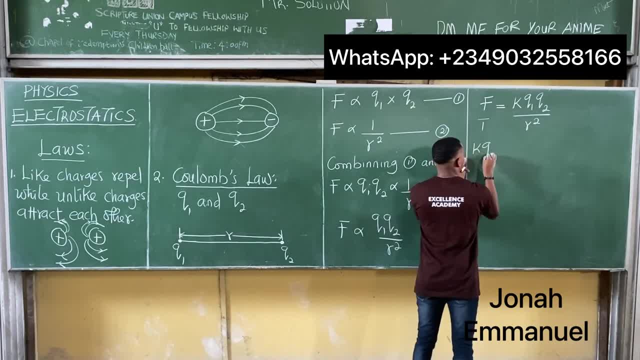 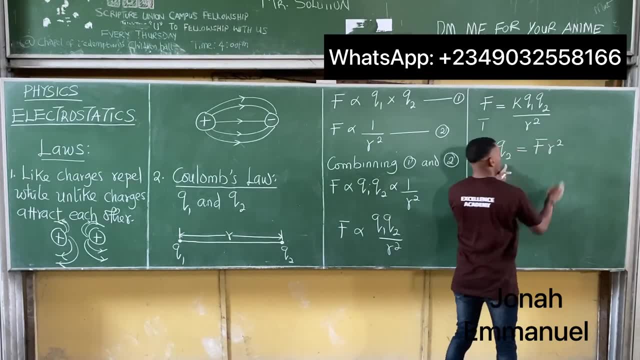 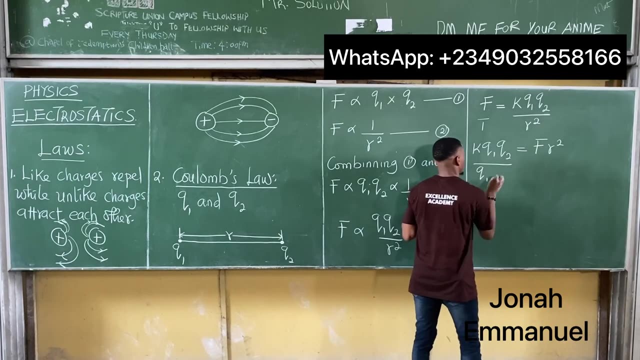 So this times 1 gives you K Q1, Q2 equal to This times gives you F times R squared, That's F R squared. So I have this To make K something good. divide here by Q1, Q2.. 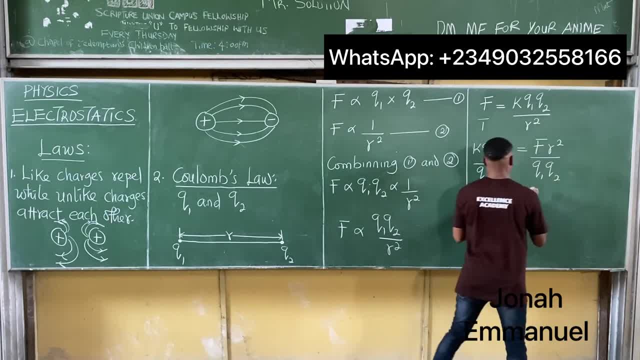 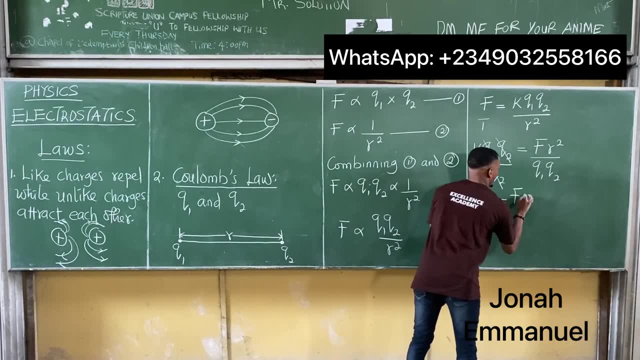 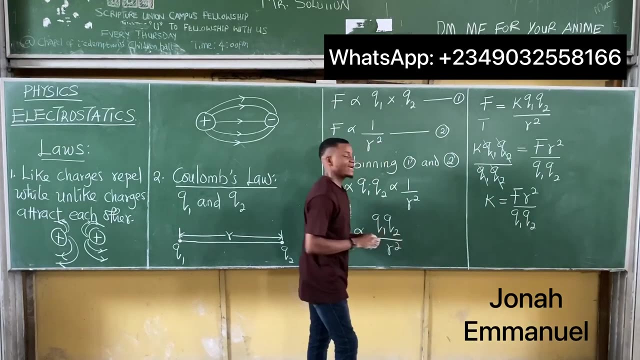 Divide here by Q1- Q2.. From here we have this K. This comes to this. This comes to this. It's equal to F? R squared all over Q1- Q2.. Alright, Let's get the SIU of the constant K. 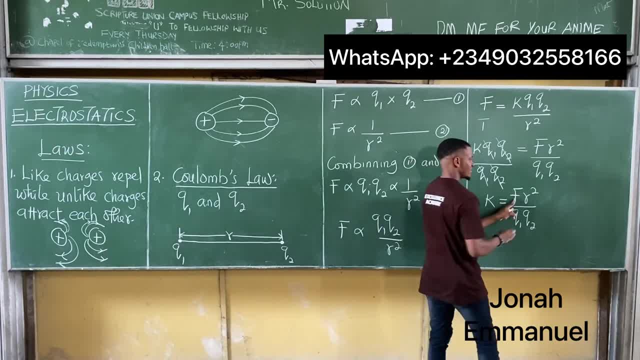 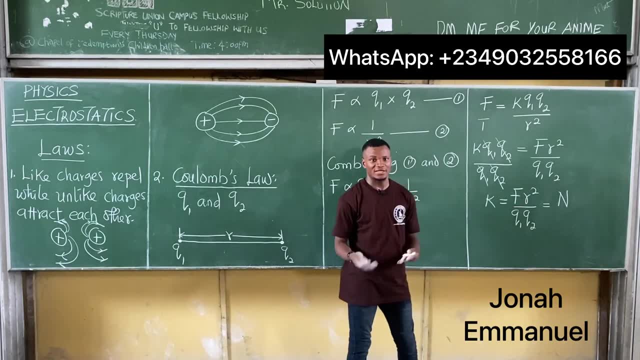 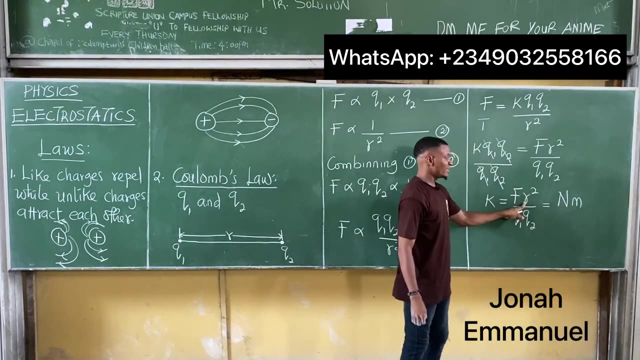 The SIU of the constant K will be: This is force. Force is measured in Newton. This is distance of separation between charges, And distance is measured in meters. So R is measured in meters. But okay, Time is being squared. 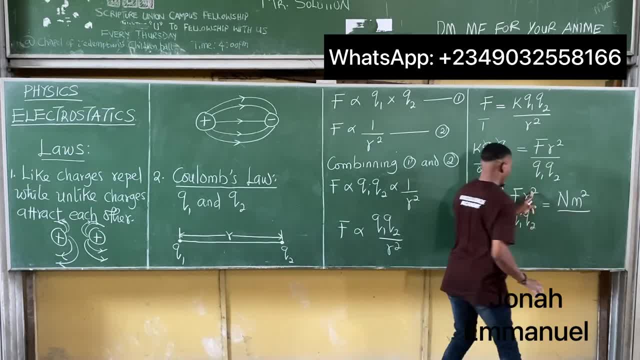 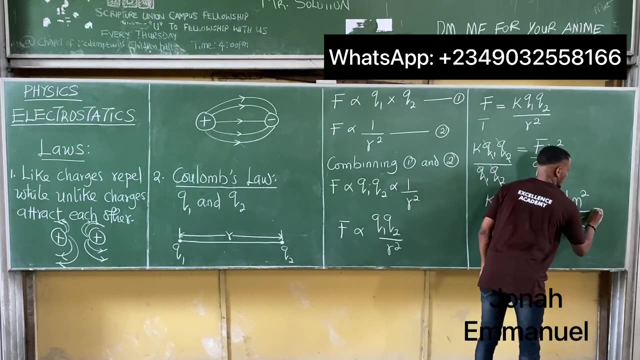 So it becomes meter squared all over. Q is charge. Charge is measured in coulomb. It becomes coulomb. It becomes coulomb. That's for this Time is under coulomb. for this This is equal to Newton meter squared all over coulomb squared. 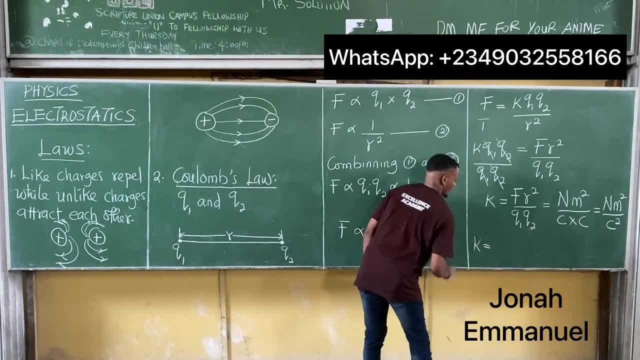 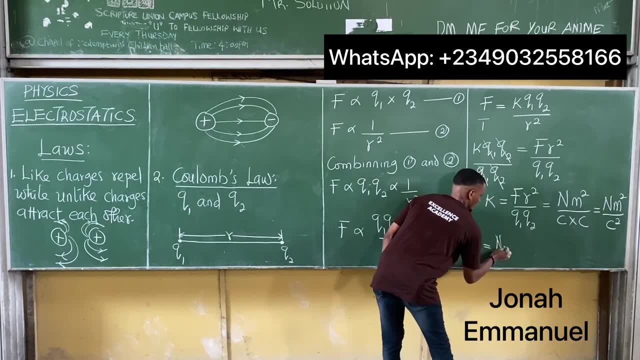 So we have this From this. K is equal to. If I draw this in index form, This becomes Newton meter squared: Newton meter squared times 1 all over coulomb squared. Is it correct? Because Newton meter squared times 1 gives you Newton meter squared all over coulomb squared? 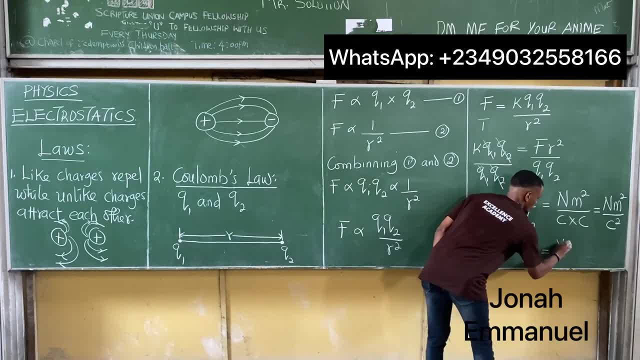 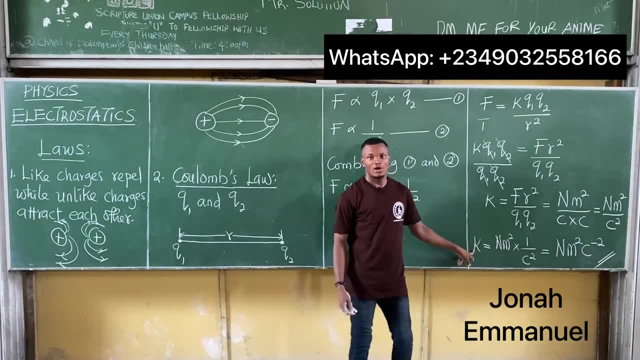 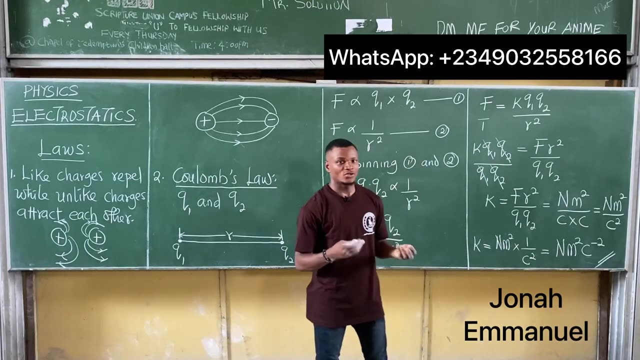 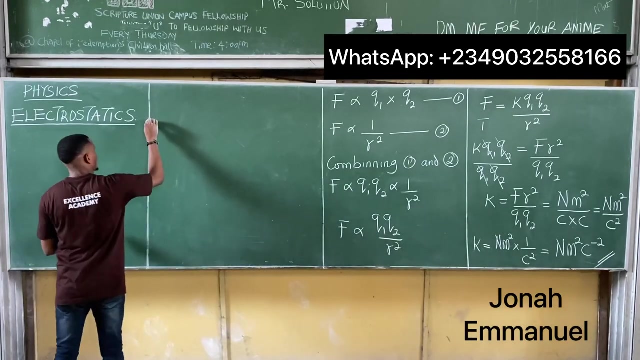 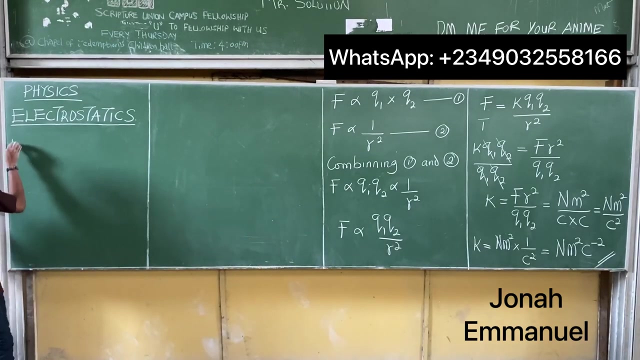 This, in index form, becomes Newton meter squared. And then this, So hence The SIU for the constant of proportionality is Newton meter squared per coulomb squared. Now, that's worth to note Also. note that, Alright. So also note that the value of K is equal to. 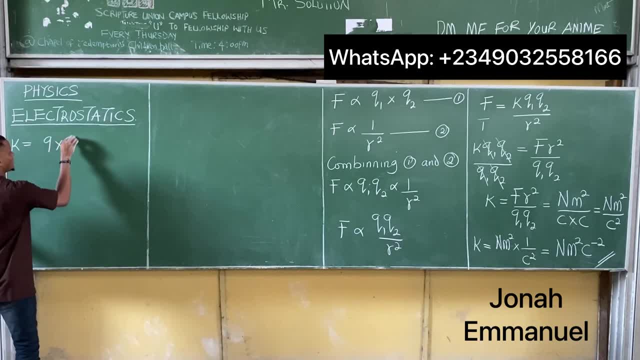 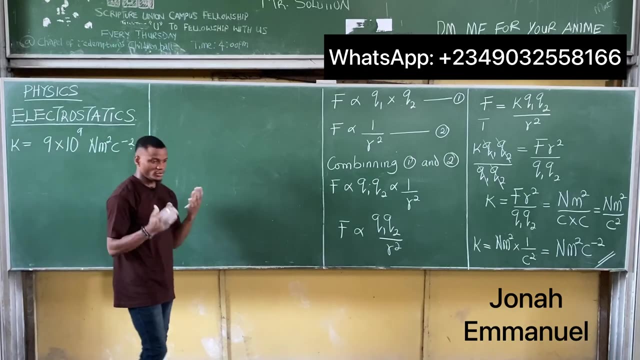 It has a constant value as 9 times 10 over 9.. If I keep it, It becomes Newton meter squared To get coulomb squared. So this becomes whatever. here. Also Experimentally, The Relationship between K and permittivity of free space is given by half the half. 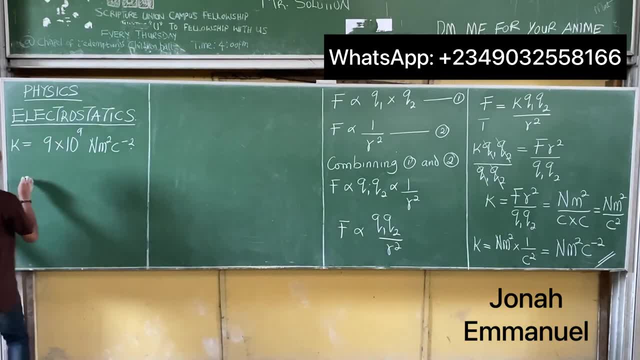 You can see, We can express K as being equal to 1, all over 4. pi E naught, We have E naught, We are also equal to 1.. Now, Well, So here A0 is equal to a constant of proportionality called connectivity of these things. 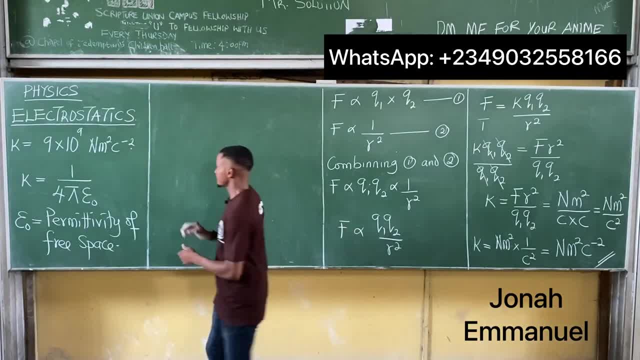 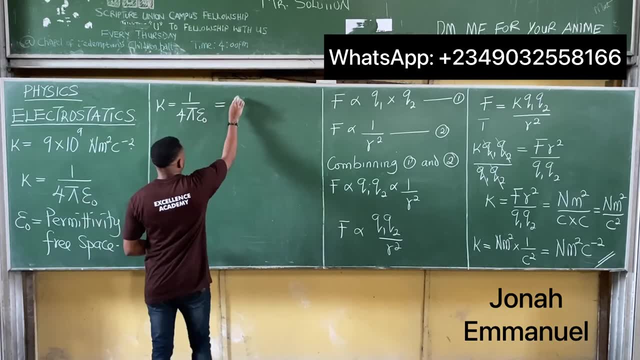 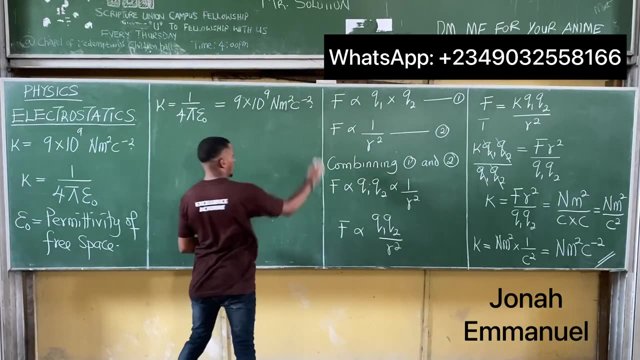 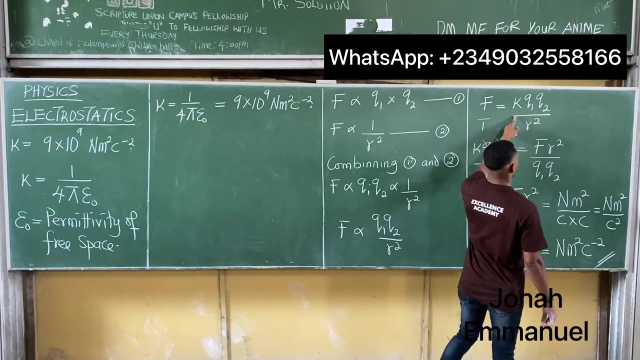 So here is equal to 1, that means K is equal to 1 over 4 pi A0, and its value is 9 times 10 to the power, 9 meters per second squared. Alright, so, having said this, if I should write this equation in terms of this: 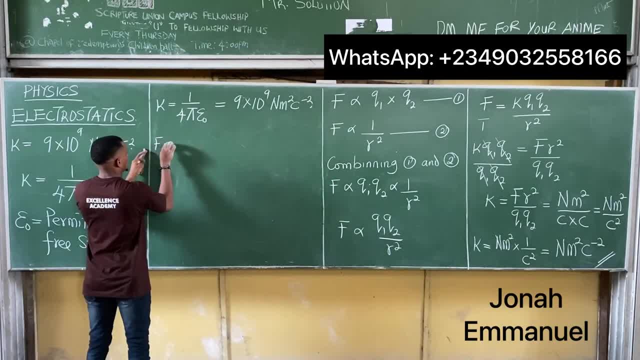 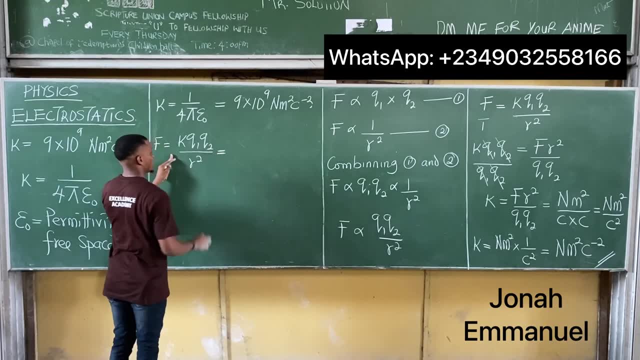 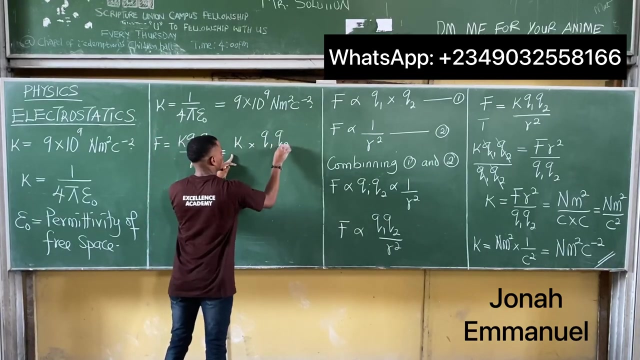 it means that F is equal to K, Q1, Q2 all over pi squared. That's equal to about K, We said We said K itself, or we have to simplify it. Shift K out of this becomes K times Q1, Q2 all over pi squared. 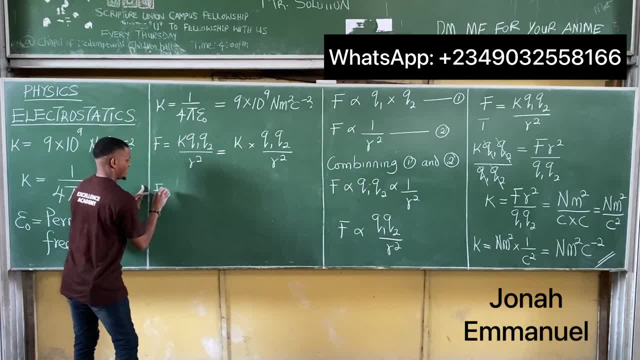 We said K is 1 over 4 pi A0. So F is now equal to K, 1 all over 4 pi A0. So K times Q1, Q2 all over pi R squared. Combine this so you can see F is equal to 1 times Q1. Q2 gives you: 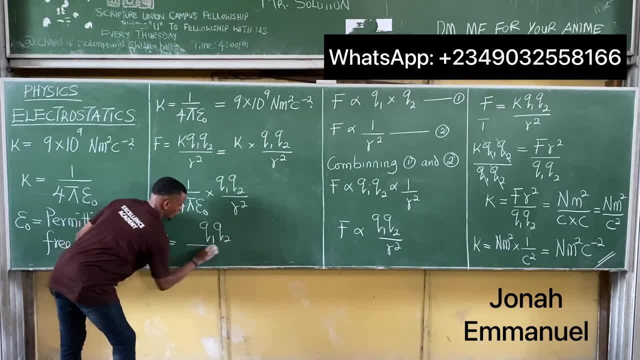 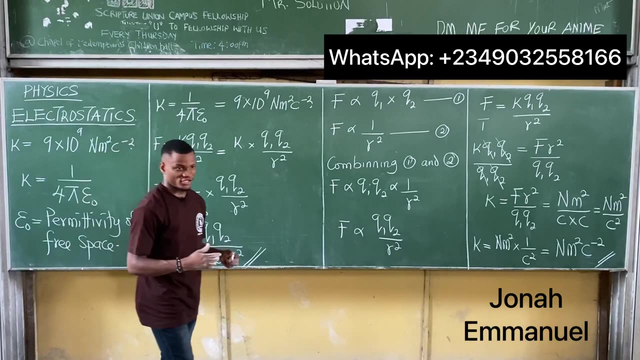 Q1- Q2 all over. this times this 4 pi A0 R squared, So we have this Alright. so here comes the formula for the Fritzi Laplace: F equals to Q1- Q2 all over 4 pi A0.. 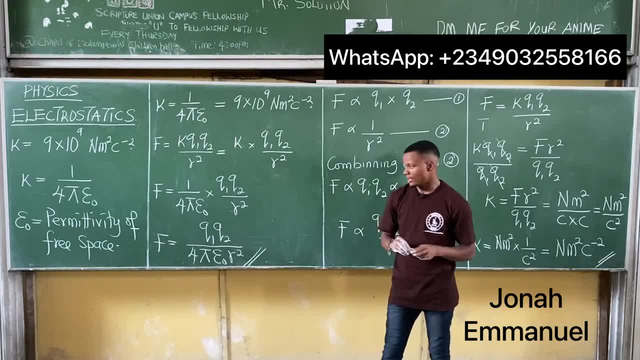 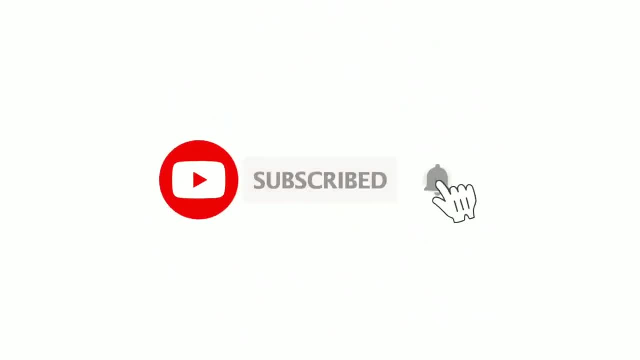 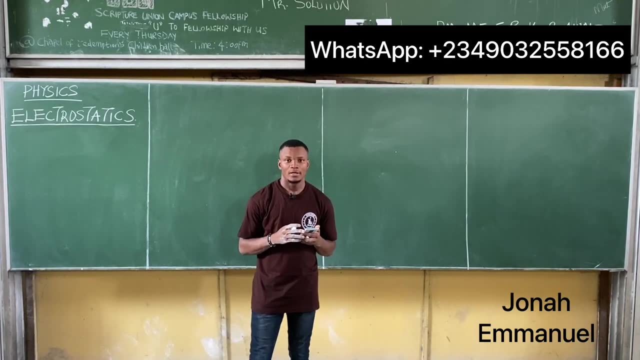 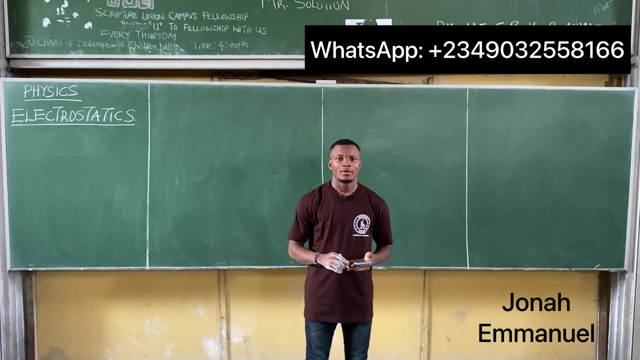 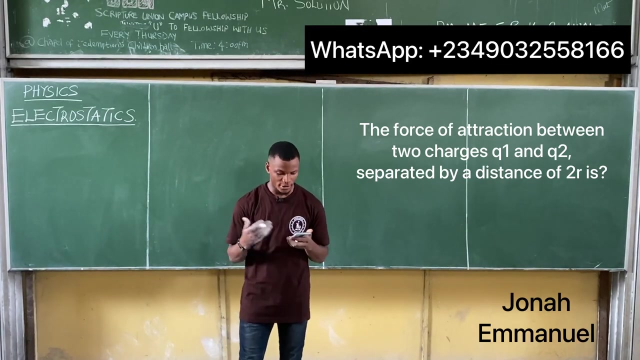 Of course it's in Newton, So let's look at some problems of relative status from what we've done so far. The first one says the force of attraction between two charges, Q1 and Q2, separated by distance. 2R is given by dash. 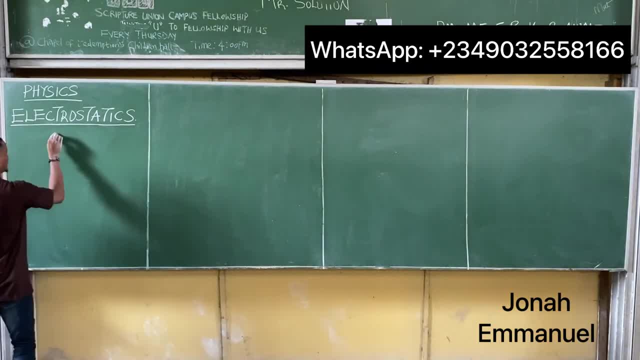 Alright, let's get this done. So solution: it gave us the charges as Q1 and Q2.. Let's say this point here: Give us this as Q1 and Q2.. And it says separated by distance of 2R. 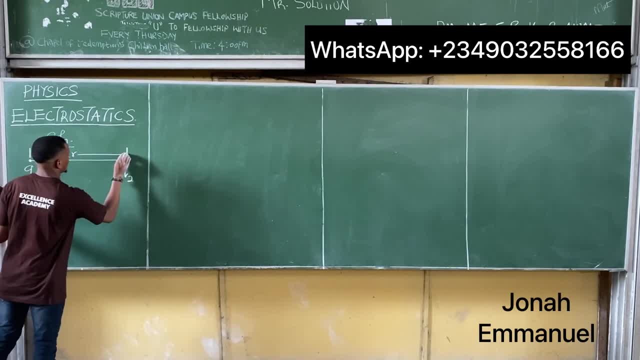 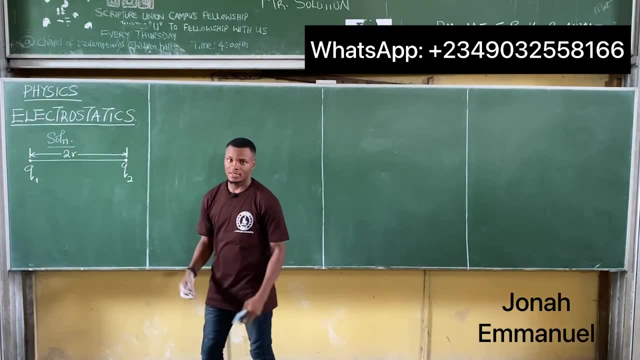 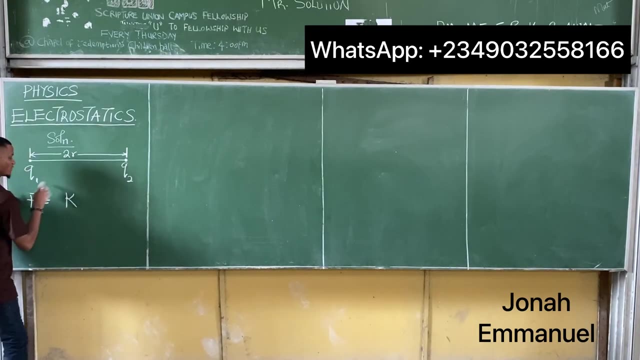 So from here to here is 2R. So to find the expression for the force of attraction between these two charges, Well, it's simple enough. We say: F is equal to K times product of charges Q1, Q2, all over. 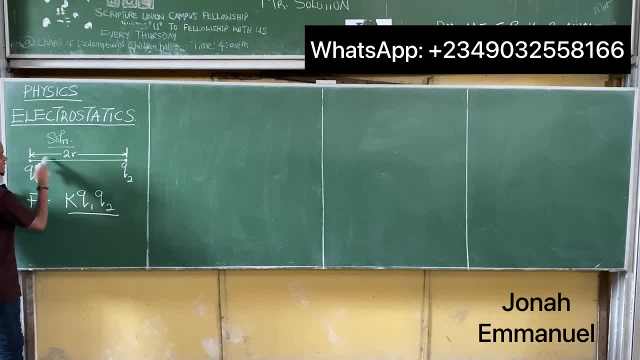 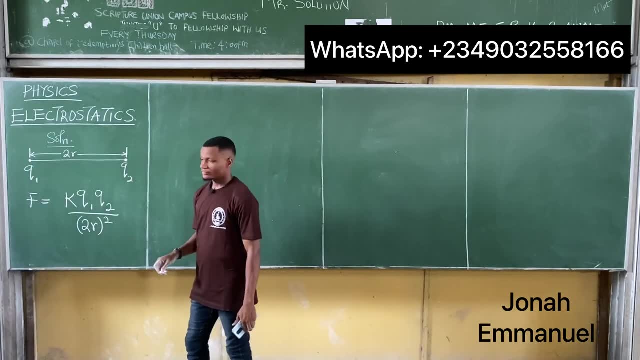 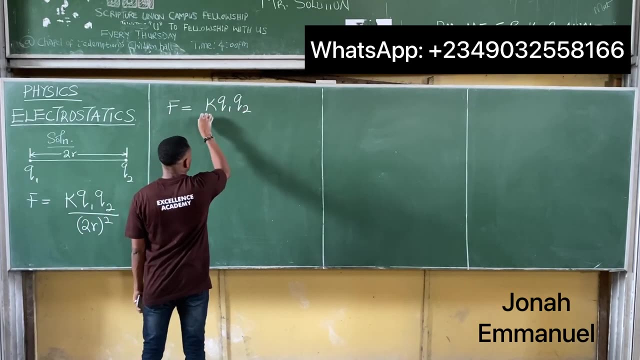 square of distance apart. Distance apart of this becomes 2R, Please, all square. So this square affects everything here. So hence F is equal to KQ1, Q2 all over, So this square goes to 2.. That gives you 2 square. 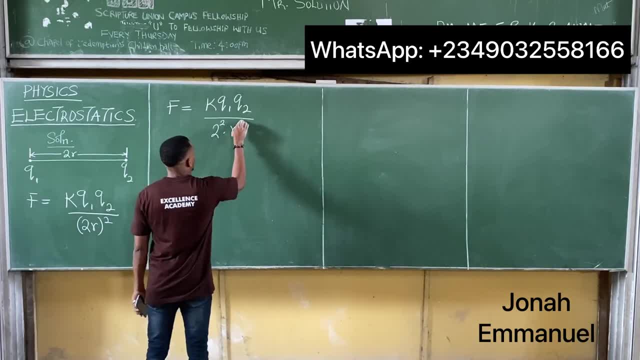 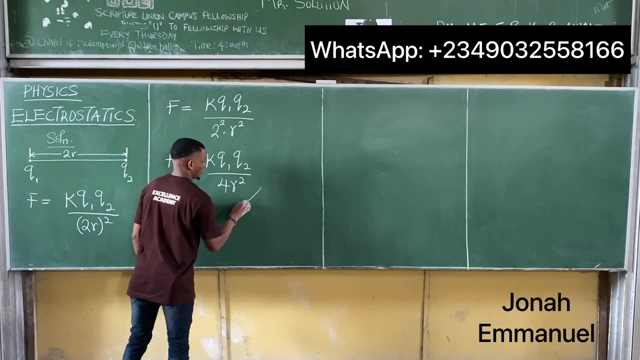 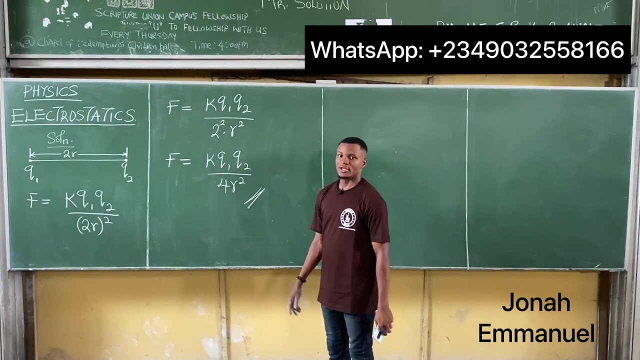 But square goes to I, That becomes I square. So F is equal to K, Q1, Q2. all over, 2 square is 4.. That gives this R square. So this becomes the expression for the force between two charges, Q1 and Q2, separated by distance, 2R apart. 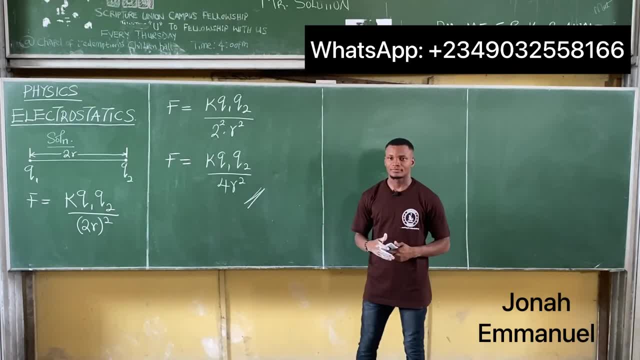 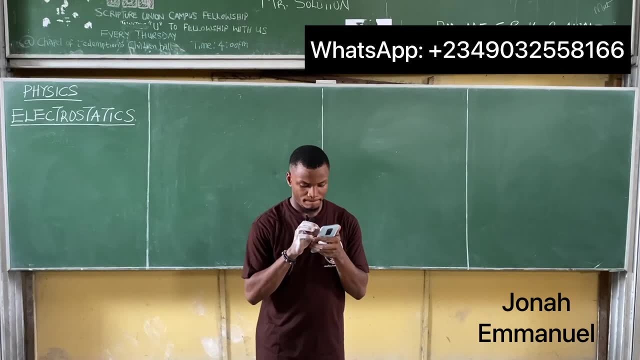 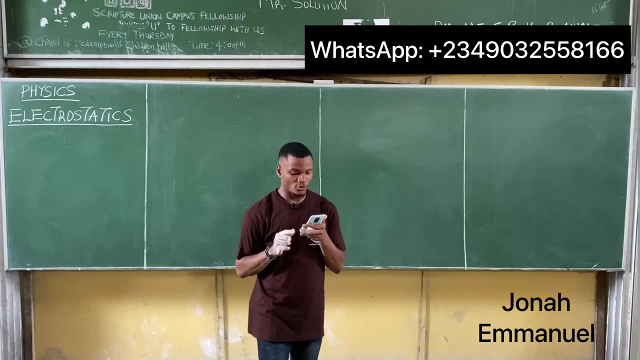 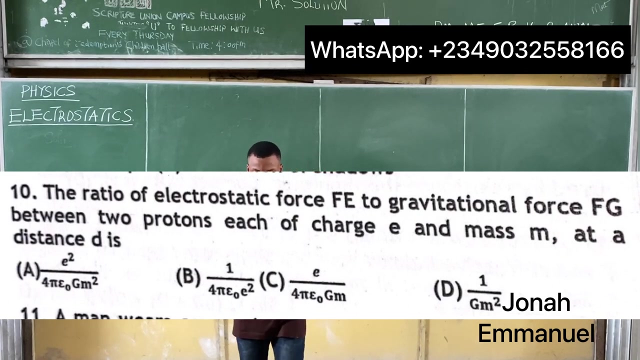 So this is the solution to that question. This question says the ratio of electrostatic force Fe to gravitational force Fg between two protons each of charge E and mass m at a distance d is dash. So how do we get this done? 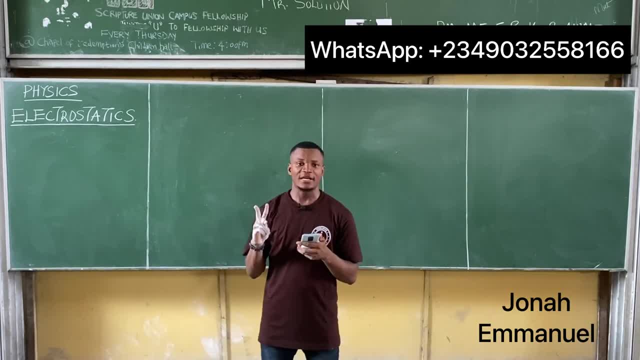 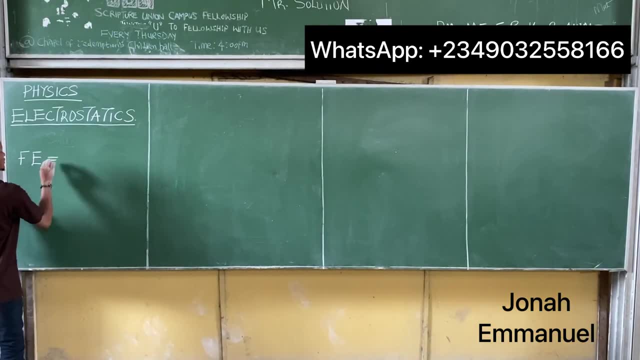 Now, before you solve this, consider something here. Two things have been given there. Number one, electrostatic force, that's Fe, is set for two protons of charge E, So that would be K. yes, hold on, how far now. 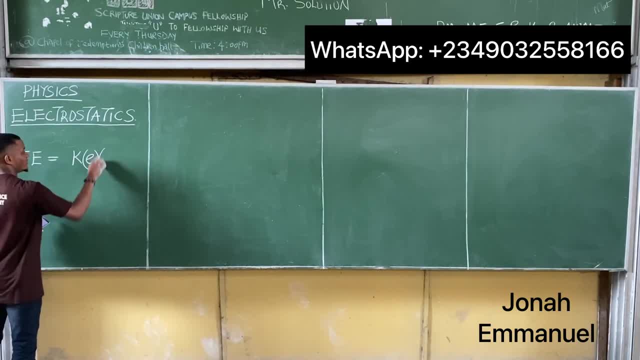 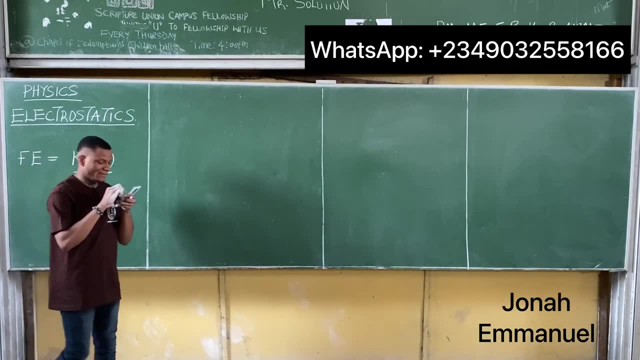 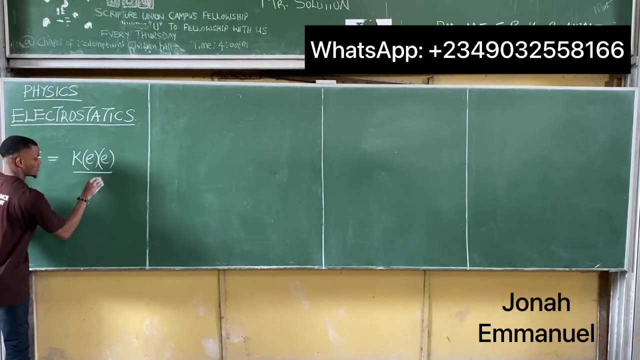 K. my first charge would be E. My second charge would also be E. So K, Q1, Q2, all over. They said the distance apart here, at the distance d my distance apart here becomes d, So d square. 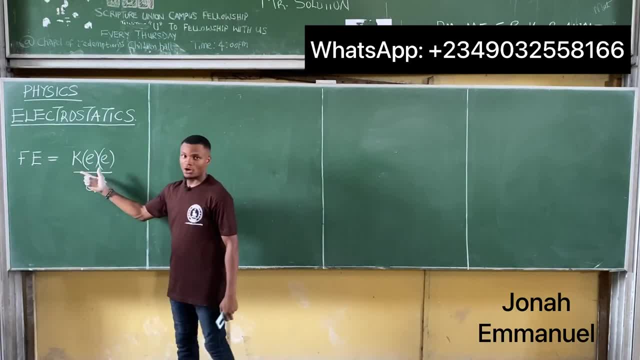 So this is the same idea of K, Q1,, Q2, all over R square, But here we're using E as a charge and not just Q. Alright, also, the distance here as given in the question, was d, not R. 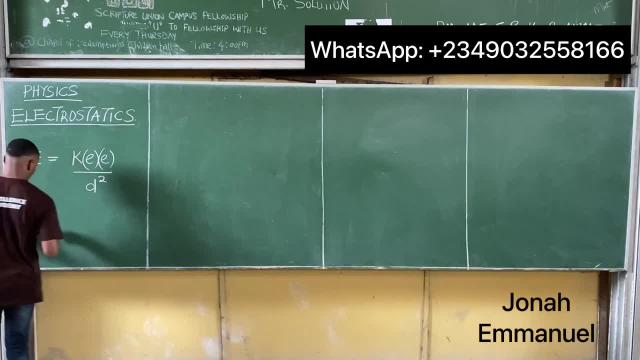 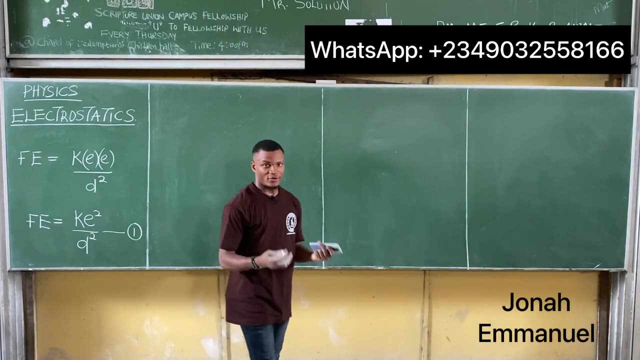 So we're using d again, But the same concept. From here, the electrostatic force Fg is equal to K E times E. is E squared all over d squared? Call this the expression for electrostatic force. Next up, let's look at expression for gravitational force, Fg. 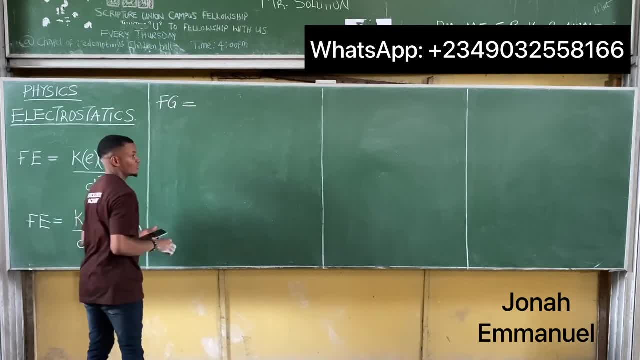 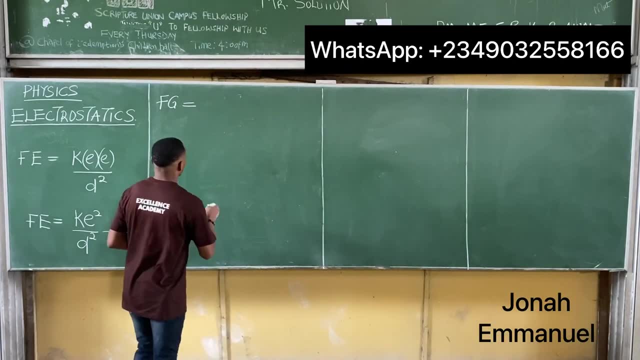 Fg is equal to now. we said for gravitational force, which we've dealt with previously, we said this one deals with masses. Alright, So we call G of M1, M2, all over R squared. This is from. 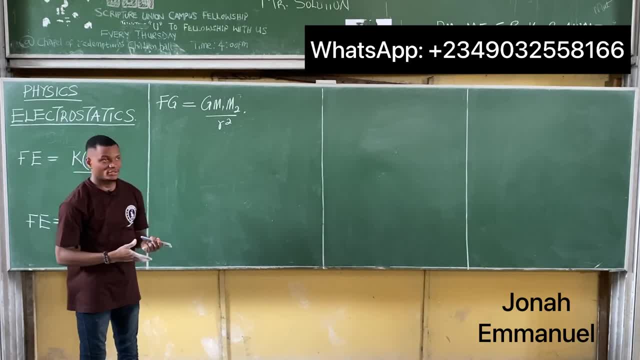 uh, gravitational law of attraction between two masses. Alright, so this is the formula. It's very similar to electrostatic force, But the difference is that for electrostatic force it talks about charges, while it talks about masses. For electrostatic force, 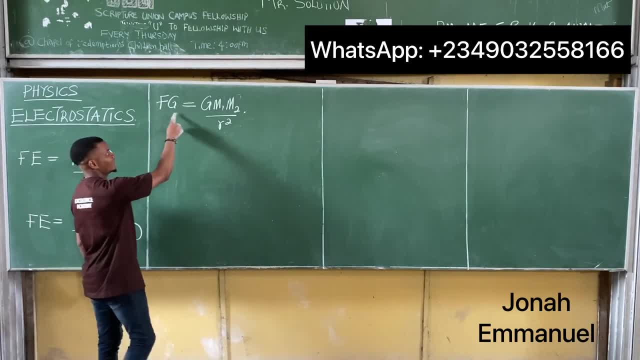 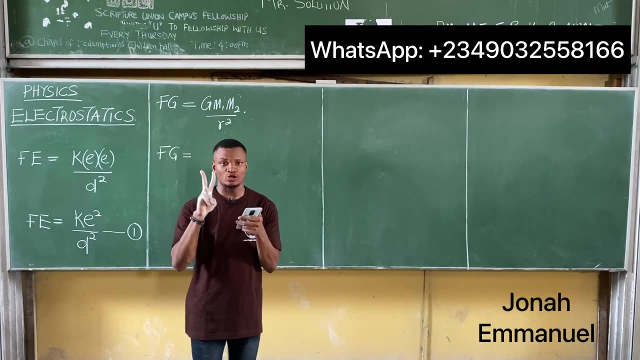 you have K as a constant. For this, we have G as a constant. Relating this to a given question: for the question we said Fg is equal to, we said it has a ratio of okay between two protons. 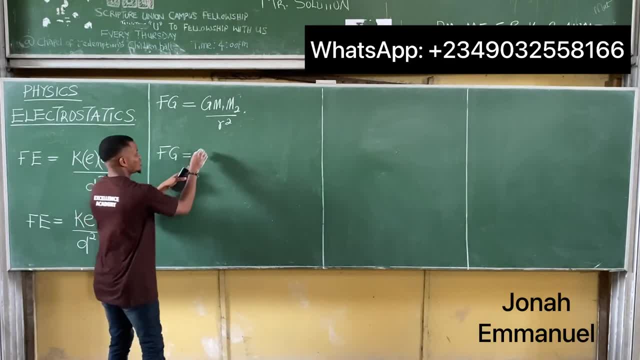 the two protons, the cell of mass M to become G. Just as we have similar charges for the protons, of course we have similar masses for the protons. So it's not only that: M1, M2,. 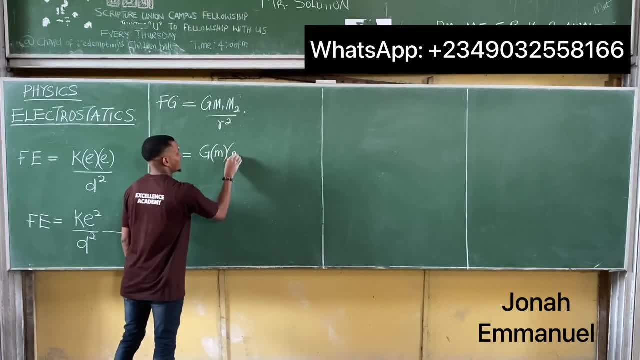 becomes M for proton 1, and then M for proton 2.. The distance of separation as given was Z for R D squared for R Z- Same concept. So this is now equal to G. 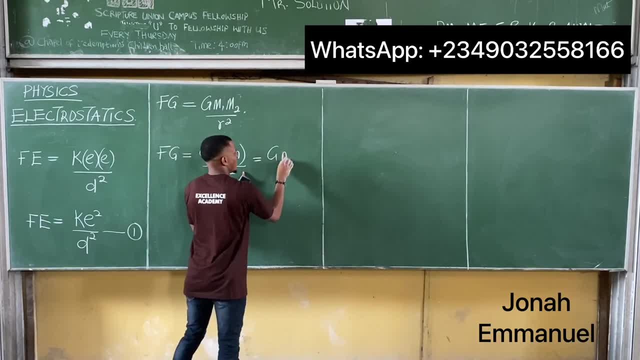 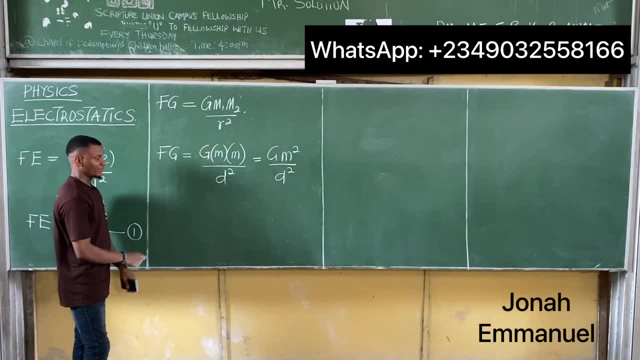 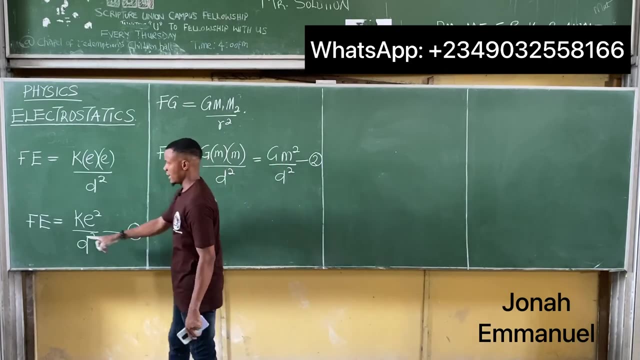 M times. M is M squared, all over Z squared, So Gm squared all over D squared. Now we have an expression for electrostatic force and gravitational force Next up. 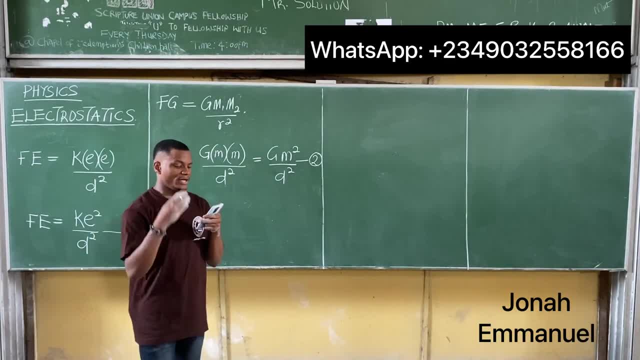 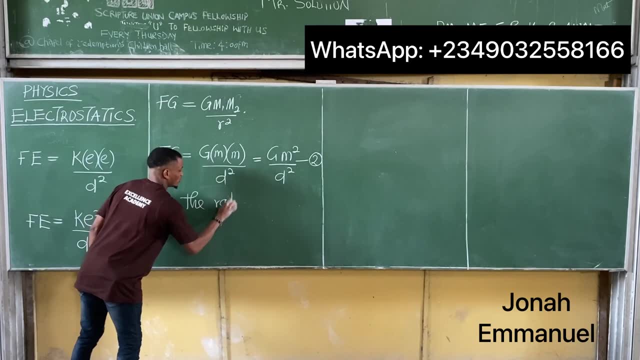 we say the ratio of electrostatic force to gravitational force. So therefore the ratio, the ratio will be Fe- electrostatic- to Fg- gravitational. Alright, If I want to be equal to. 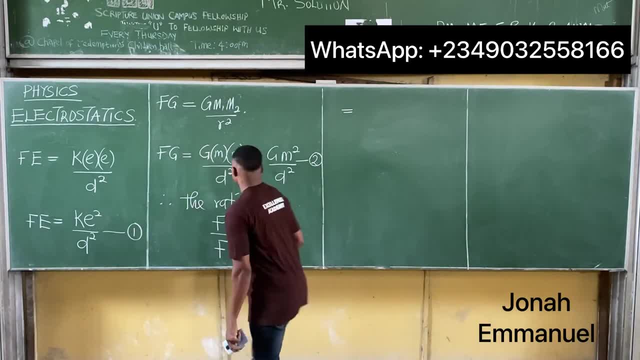 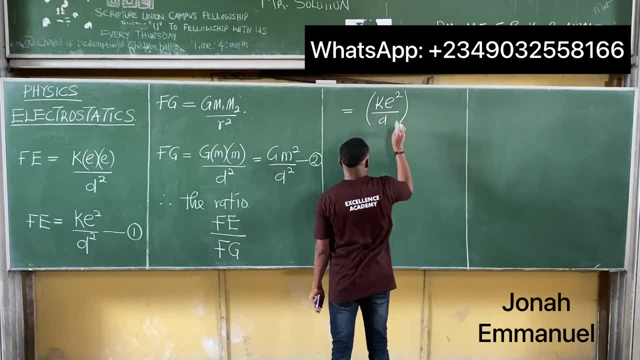 for electrostatic. I have this: it becomes K E squared. all over D, all over gravitational. I have this becomes G M squared. So all over D squared. Yeah, Alright, So. 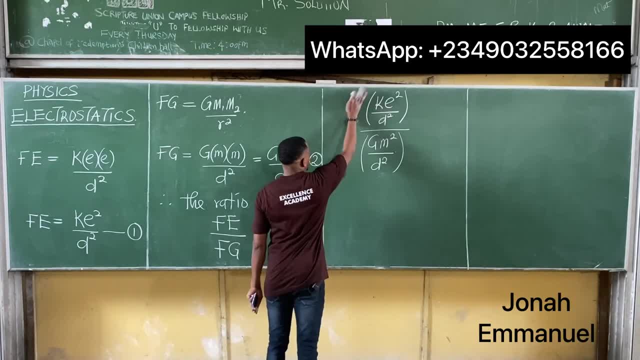 Gm squared, all over D squared. So I have this, And electrostatic force to gravitational force. I have this. I will break this down and work it up, So this can't be to simplify it. 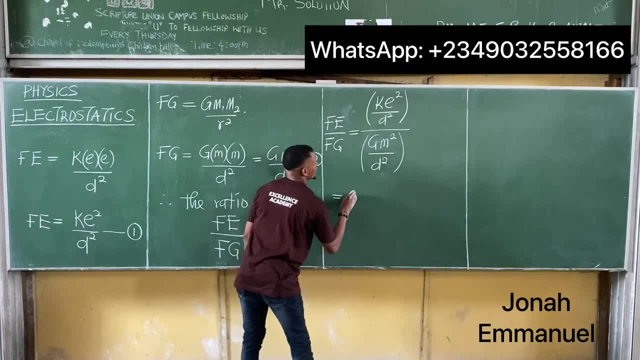 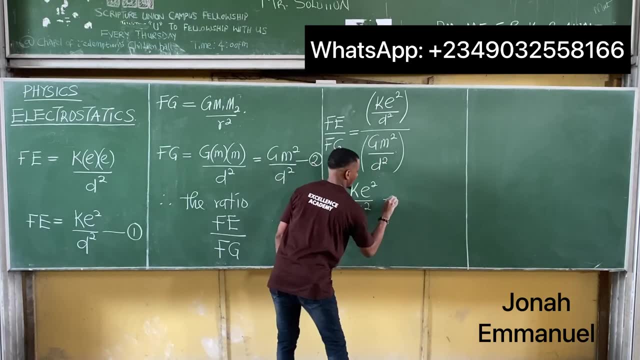 We can write this as saying: this is equal to K. E squared all over D squared. divided by this one here, G M squared all over D squared, This will now be equal to E squared. 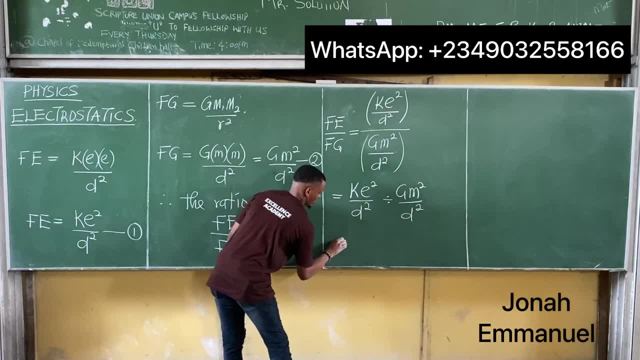 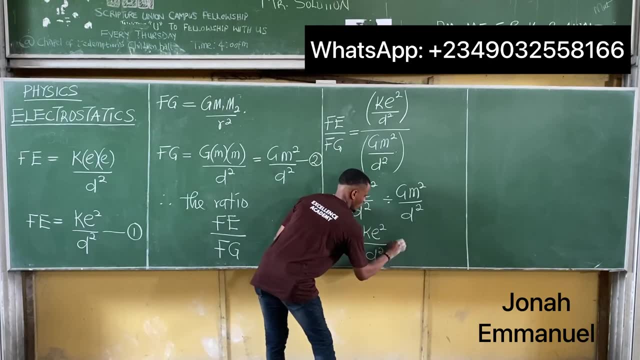 all over D squared. divided by this will now be equal to K E squared all over D squared. change here to multiplication and invert. So this is how you solve fractions, or division of fraction. 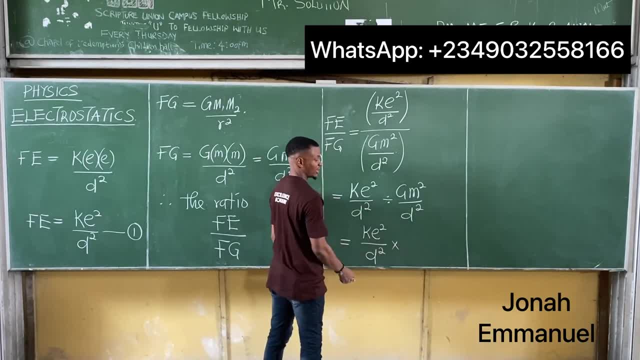 We say: change division sign to multiplication and, of course, invert this. So that's how you solve this. It becomes D squared all over G, M squared From here. this will cancel this. That is equal to. 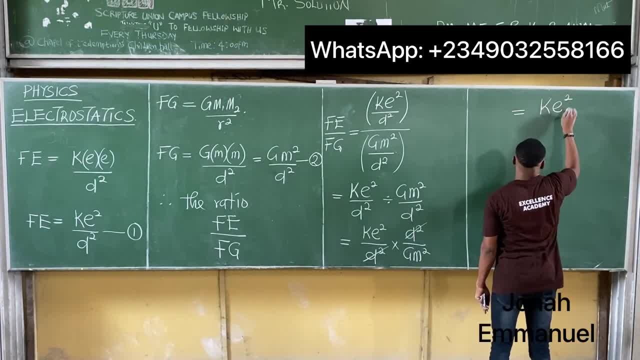 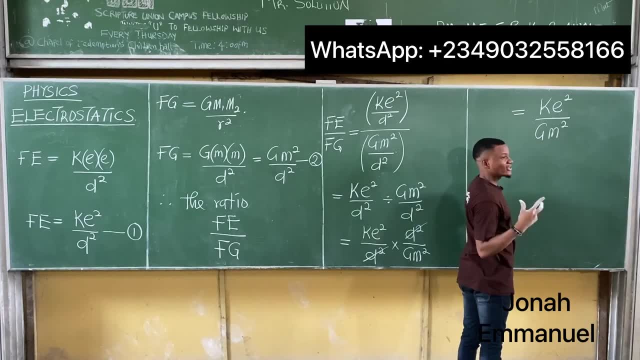 K, E squared, all over G, M squared. Of course this is charge, It cannot cancel mass, It can't cancel. This is K, It cannot cancel, G, It can't cancel. So this becomes the ratio of: 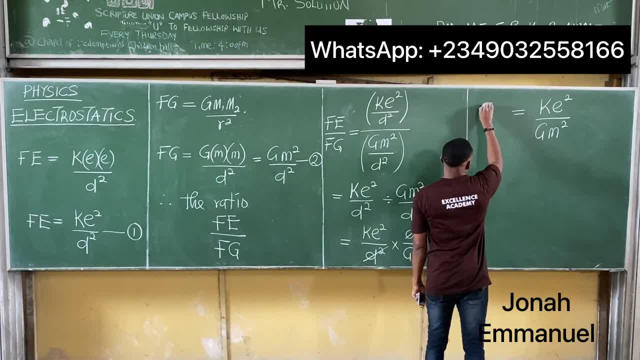 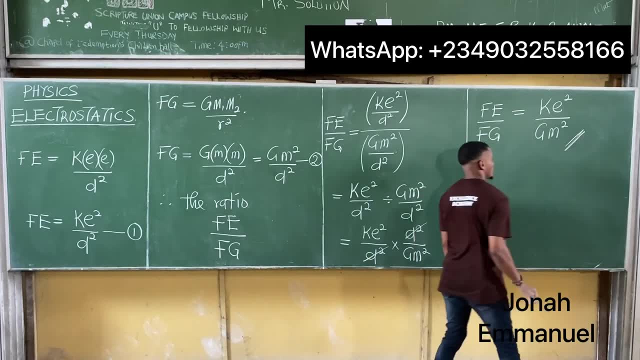 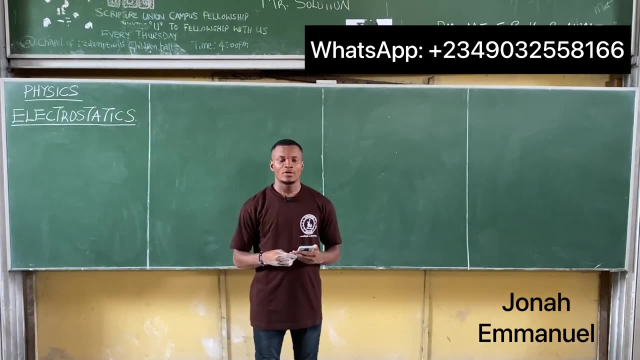 the electrostatic force to the gravitational force. So this is how you solve this particular case here, Thank you. So let's try yet another example of electrostatic. So the question is: what is the force of attraction? 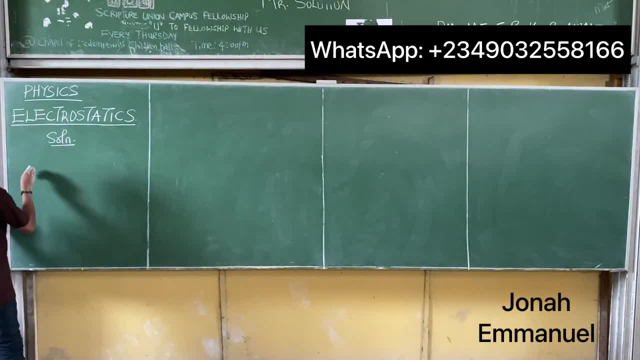 between two charges, Q1, equal to 5 microcouple, and Q2, equal to 7 microcouple, separated by a distance of 15 millimeters apart. Take one over. 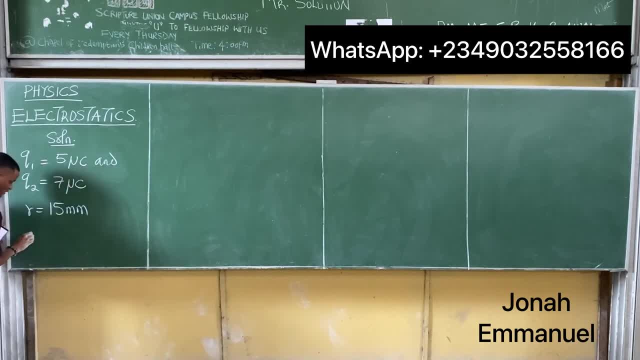 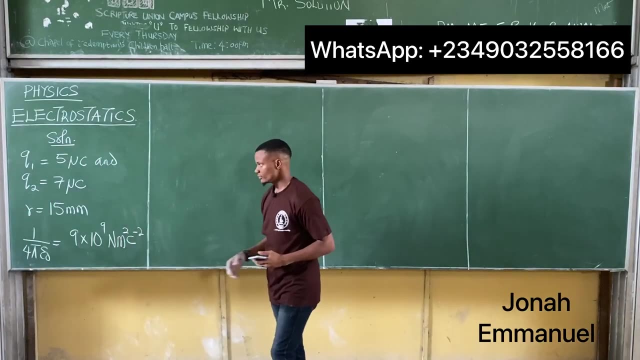 four, five in the distance of 15 millimeters. four, five in as nine times, ten times nine Newton meters square per coulomb square. Alright, so we have. 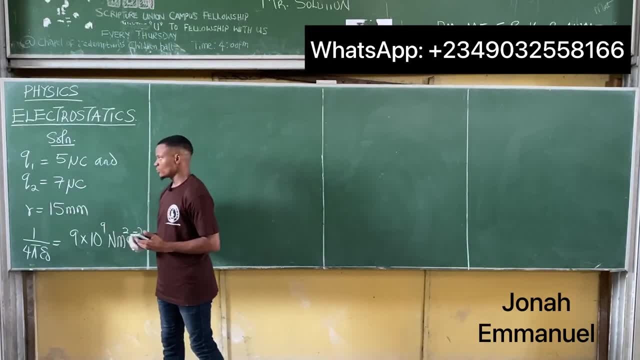 this particular distance, I'm giving Q1, as 5 microcouple, Q2, 7 microcouple, R as 15 millimeters and one of 5 microcouple. 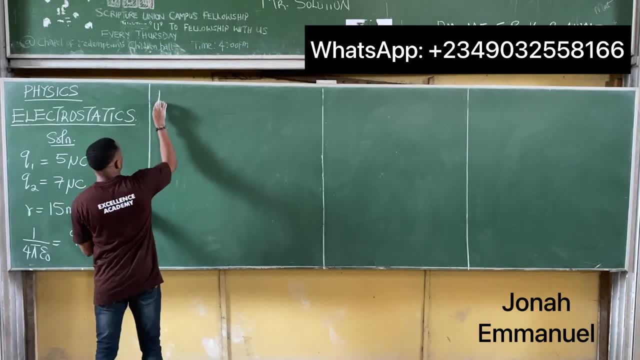 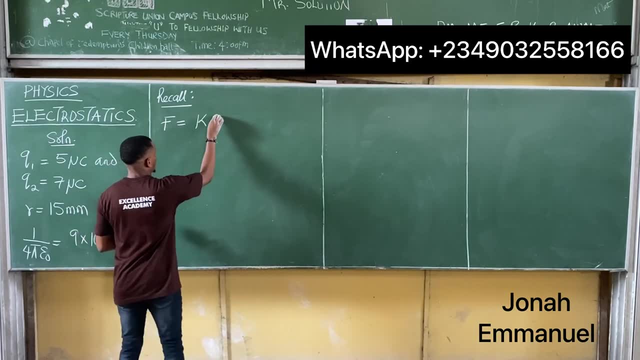 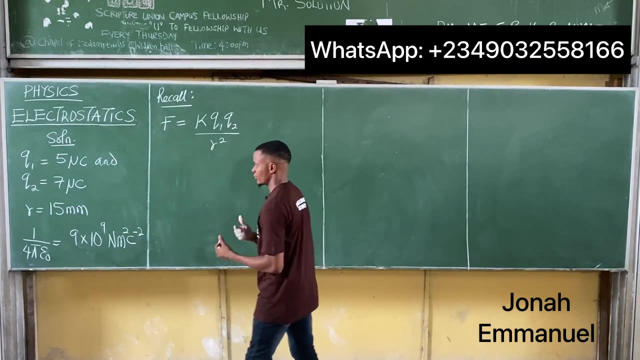 So let's solve this. So recall formula. recall that we said from coulomb's law: F is equal to K, Q1,, Q2, all of them R squared, My S, that's equal to my conversion. 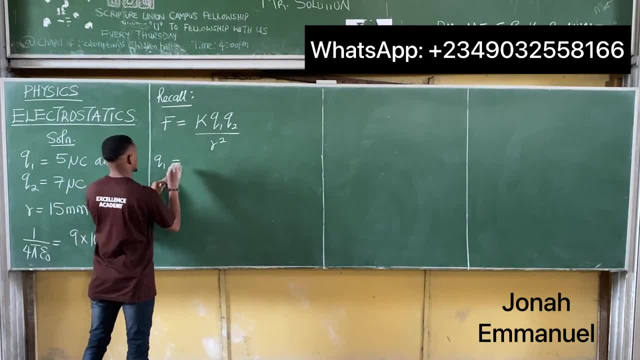 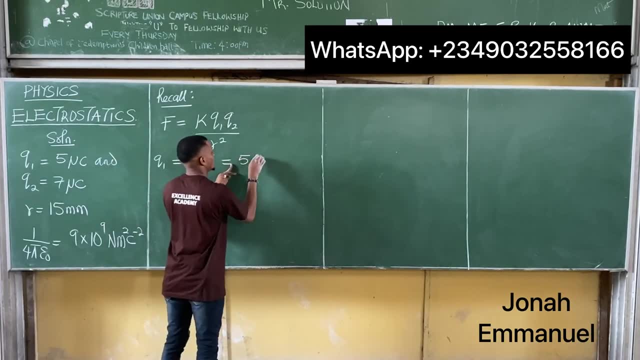 and my conversion, Q1,, we said, is 5. microcouple, that's equal to micro, is times 10, bar minus 6, coulomb, That's the first one. Q2, is equal to: 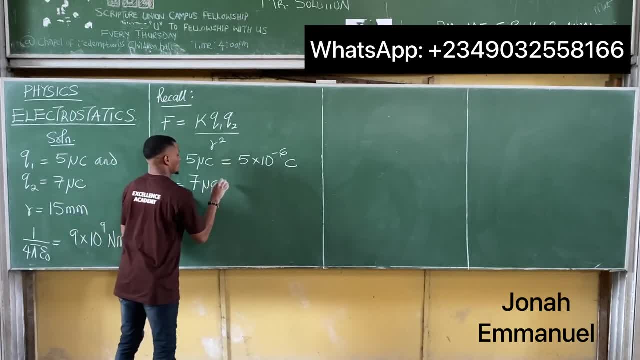 7, microcouple, that's equal to micro, is 10, bar minus 6, coulomb Next up R, so R is equal to 15, millimeters. Combine this to meters. 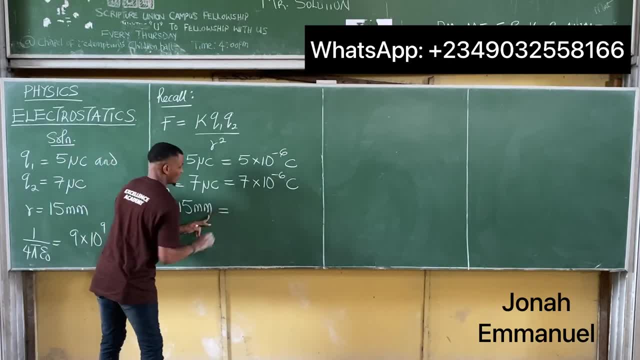 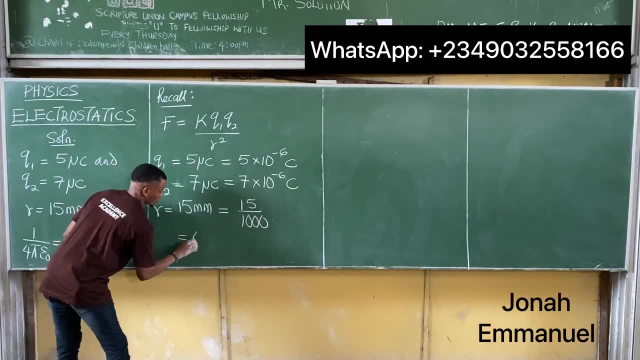 divide by 1000, and become 15 millimeters. So we come to 15 over 1000.. That's equal to 0. 0. 0. 0. 0. 0.. 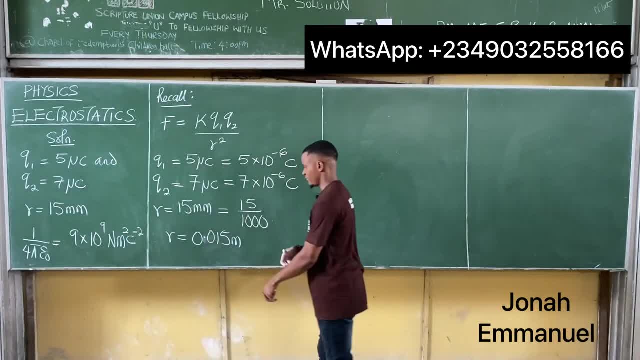 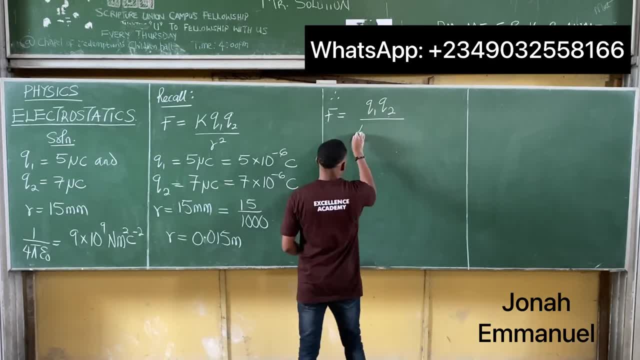 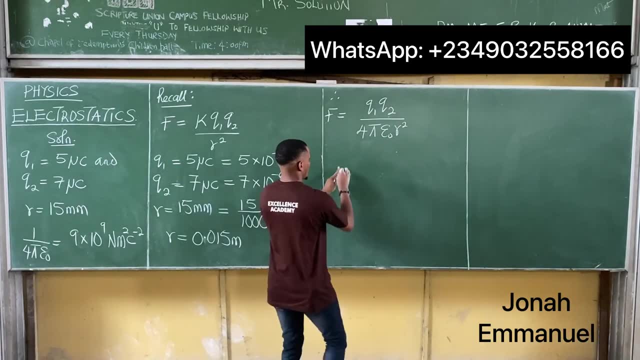 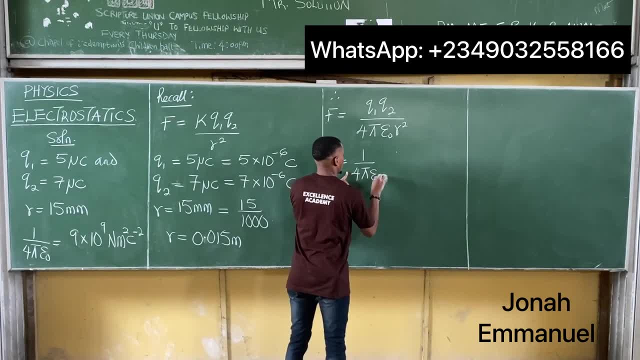 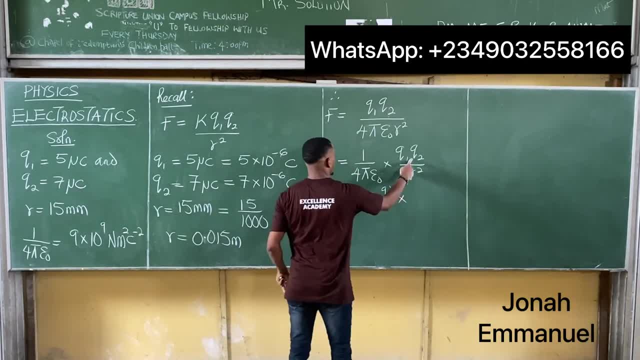 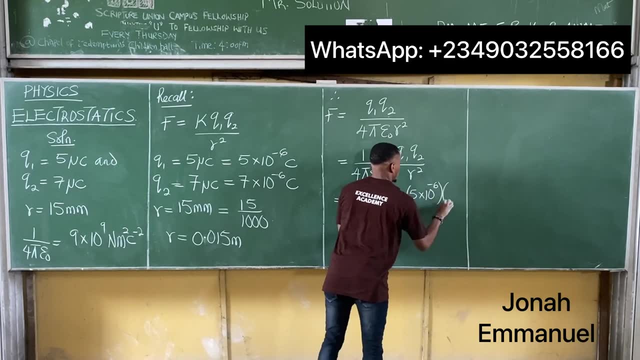